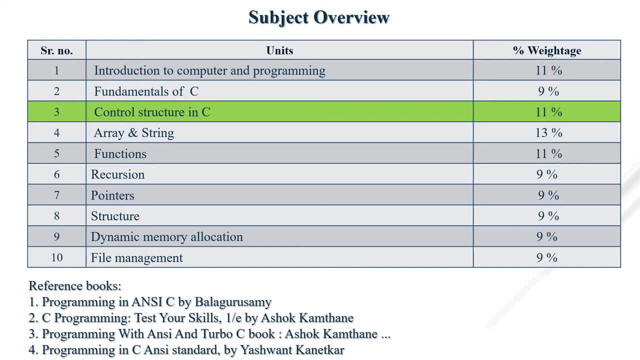 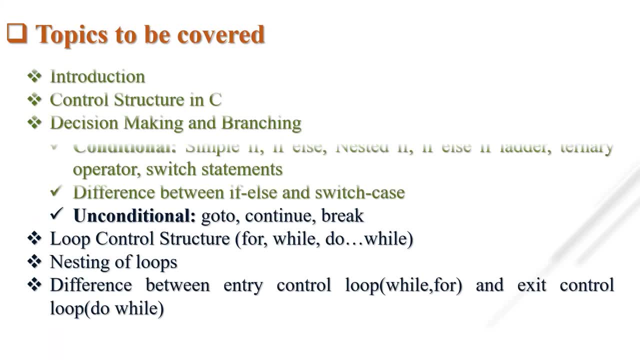 unit number 3, that is, Control Structure in C Language. So in this video the topics which are covered are Introduction, then Control Structure in C, then Decision Making and Branching, which includes Conditional Simple, if, If-else, Nested, if, If-else Indirectly, Indirectly, Indirectly, Indirectly, Indirectly, Indirectly. 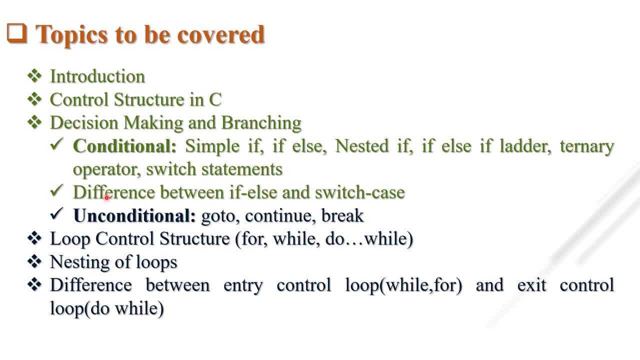 Did you notice If-else, If-later, Turnery, Operator, Switch Statement and Difference between If-else and Switch Case? So in this video only we have covered this much topic which are highlighted in green colour. Rest of the topics are covered in. 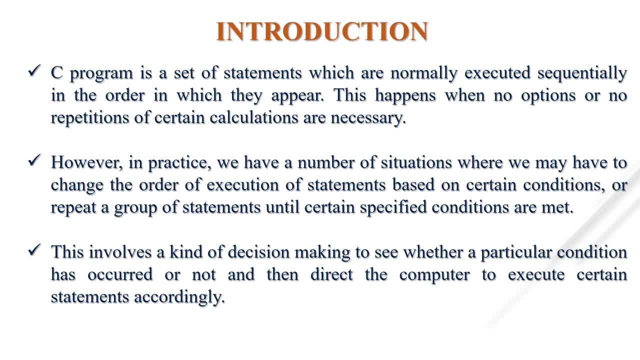 next video. So C is a set of statements which are normally executed sequentially in order in which they appear. So we know that C programming scans from top to down. This happens when no options or no repetitions of certain calculations are necessary. But in practice we have number of situations where we may have to change the order of execution of statement based on the certain conditions, or repeat a group of statement until certain specified conditions are met. 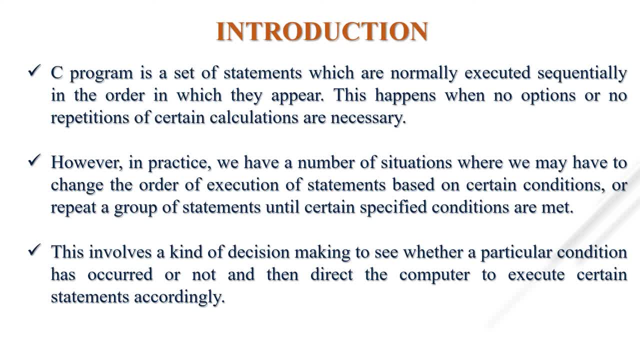 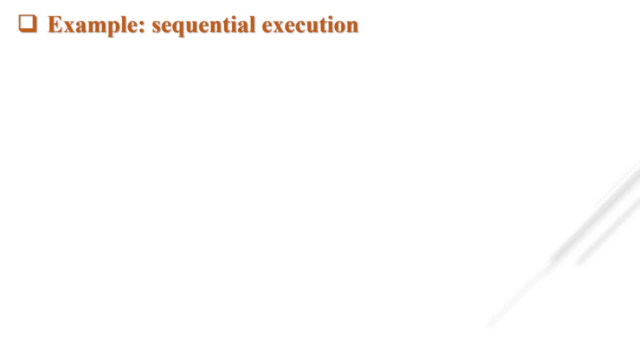 So this involves a kind of decision making to see whether a particular condition has occurred or not, and then direct the computer to execute the certain statement accordingly. So here is an example of sequential execution, where compiler scans from top to down sequentially. There is no condition in between. 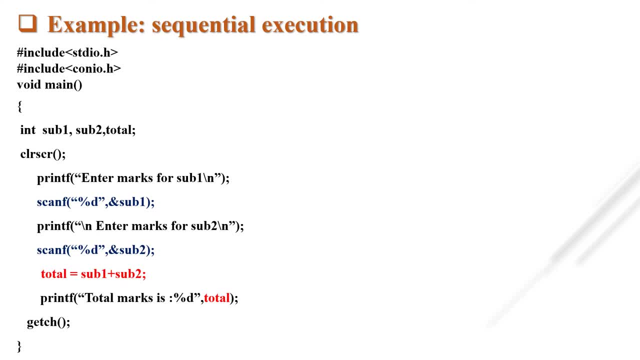 So what compiler do? It starts from top And reach to the bottom. First, there are three variables. First one is subject one, subject two and total And clear screen function will call It will use to clear the screen and output. 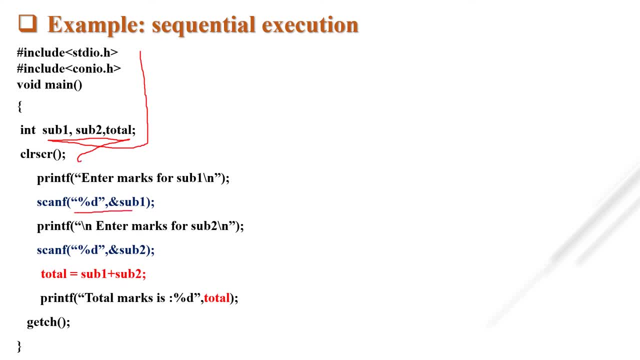 Then it takes the number which stored in subject one, And then it takes subject two max and stored in subject two variable, And then we simply total subject one and subject When the answer of this expression will be stored at stored in total. And finally we simply print. 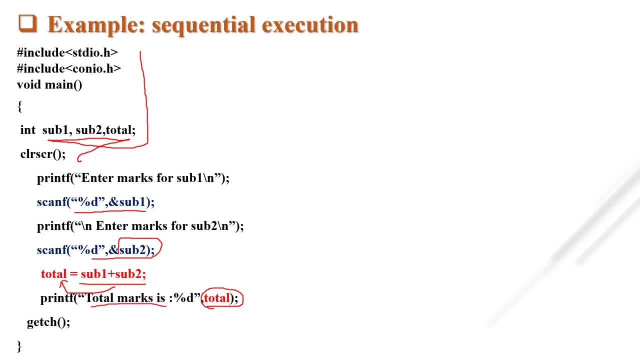 The summation of subject one and subject two at last. OK, so this program sequentially executed. in between, There is no condition. OK, from here to here. we are not going from anywhere to anywhere. So what's the output? Output is enter. subject: 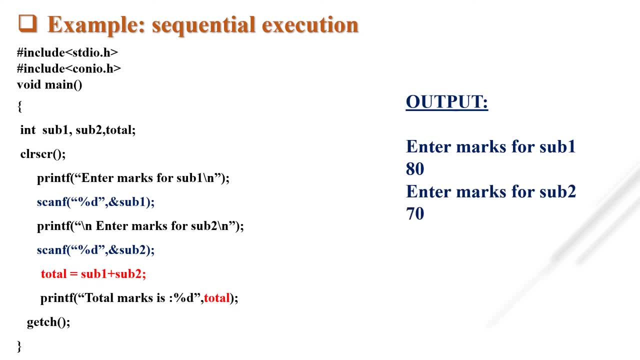 So one max: suppose I entered 80,. subject two: suppose I entered 70,, the total is 150.. So this is an simple example of sequential execution. Let's see branching. and So this is an example for decision making and branching. 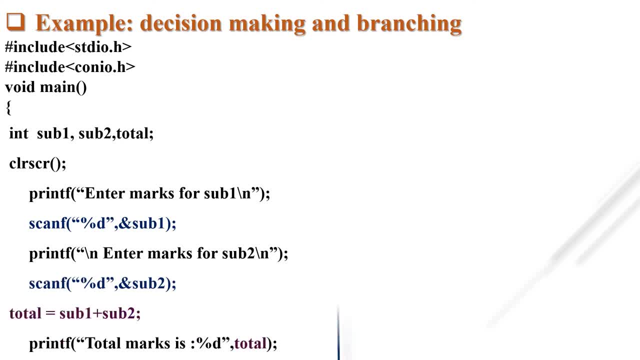 The program is not compiled sequentially. Why? Because here it is an if statement. So when if statement is true, This if statement is true, Then this part of this block will be printed, OK, and if it is false, then this block will be executed. 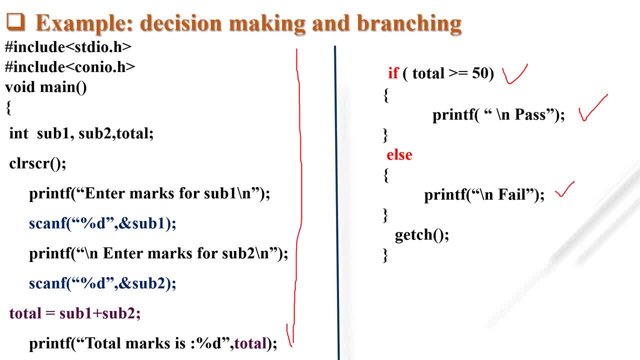 So from here to here it will be sequentially, but from here You can say: here it is a decision making And according to the condition, it will control the transfer. It may be if the total is greater than or equal to 50 is false, then the control will be transferred to the else part. 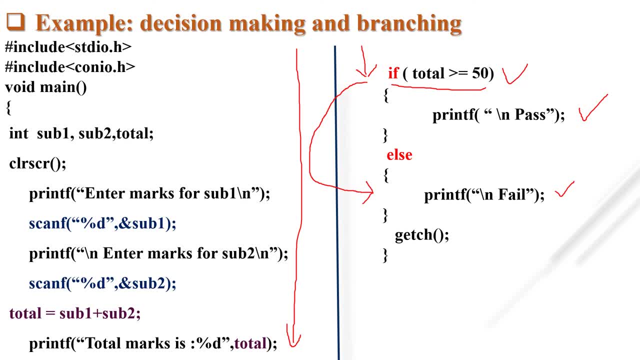 OK, so control statement are used for taking the decision and then transferring the control to the given statement. So this type of statement checks logical conditions and if the condition is found to be true, then the decision are executed. So this is the output. 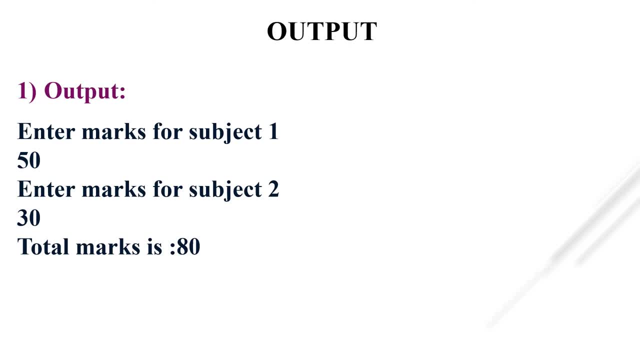 Max is greater than 50. That's what we are going to do. So this is the output: OK, Max is greater than 50.. That's what we are going to do. OK, Max is greater than 50. That's what we are going to do. 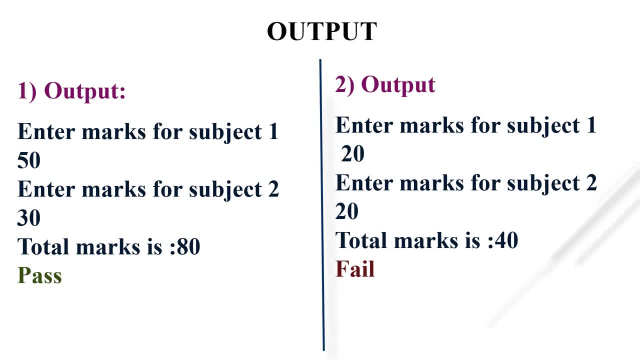 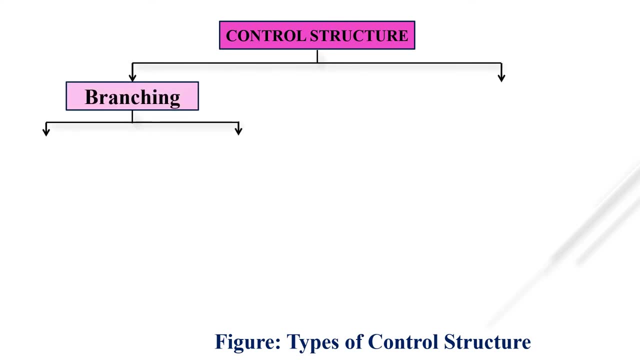 That's why it is fast. If Max is greater than less than 50, then it will be fail. OK, So this is a difference between sequential and decision making statements. So In control structure we have two types. First one is branching, which includes conditional branching and unconditional branching. 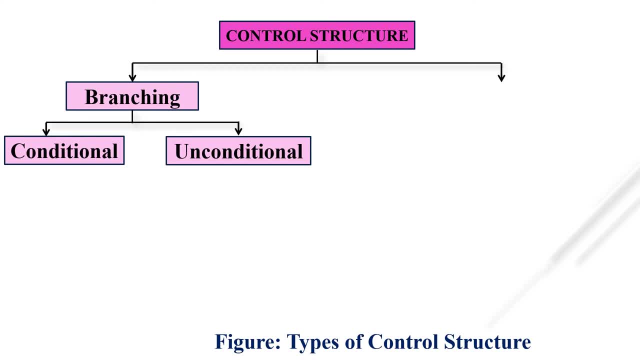 In conditional branching there are some conditions for the control statements, statements: okay. this statement checks the logic conditions and if the condition is found to be true, then the decision are executed. in conditional conditional branching includes if statement, which includes simple if, if else, nested if and if else, if later. second ternary operator that we already 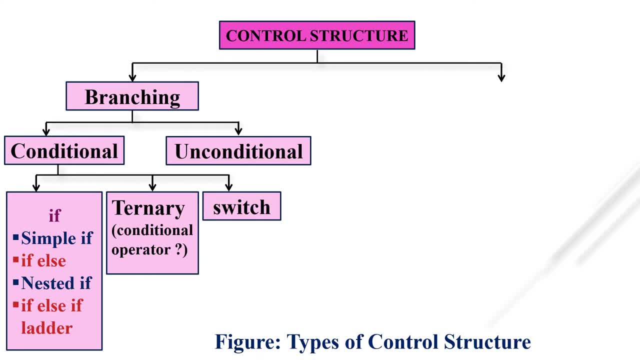 see in the previous video. and next one is switch case statement. so this three are conditional branching- okay, it has some condition to be checked, and then the control control will be transferred to that particular statement. and next one is unconditional branching, which includes go to continue and break- okay, 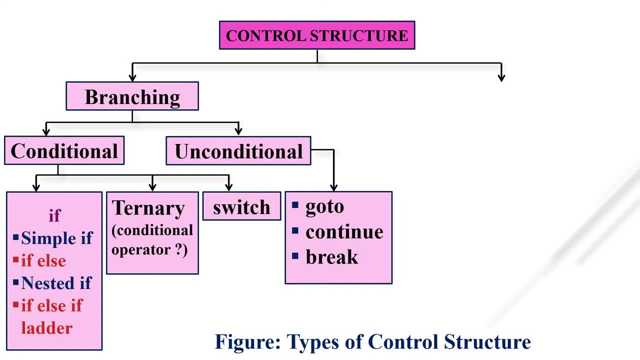 when we use go to continue and break, we don't have any condition. you can see that we have a condition, which is conditional branching, which is we directly transfer the control from one place to another place. okay, next one is looping. so these statements are used when repeated operations are to be. 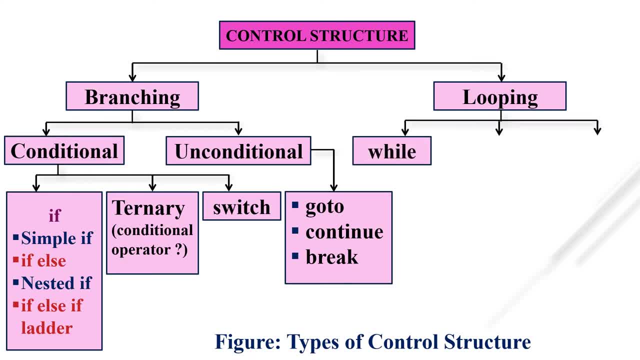 performed by iterative calculations. in these statements, loops are to be used for computing large number of values of certain variables. these statements allow us allow the user to perform the calculation of same variable with same statement, having modification of variable in the cycle till a condition is not reached to terminate the cyclic operation. so looping includes while loop. 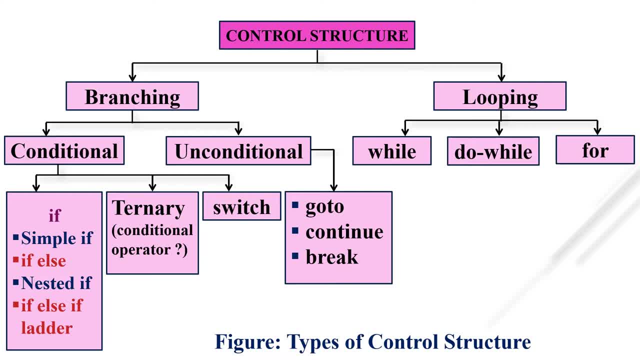 do while loop and for loop. okay, let's see one by one. first we first. we proceed with the branching in which we first come to learn what is conditional branching. learn what is conditional branching. okay, in conditional branching there are total, three statement, if statement, ternary and switch. first we go for this in: if simple, if-else nested, if-else if-lader. 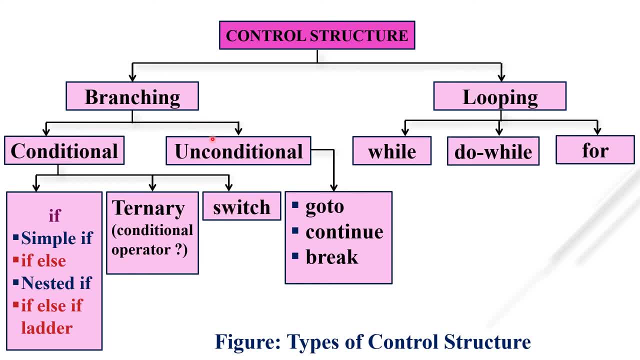 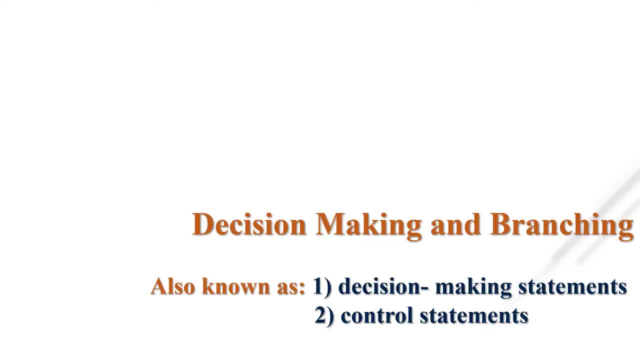 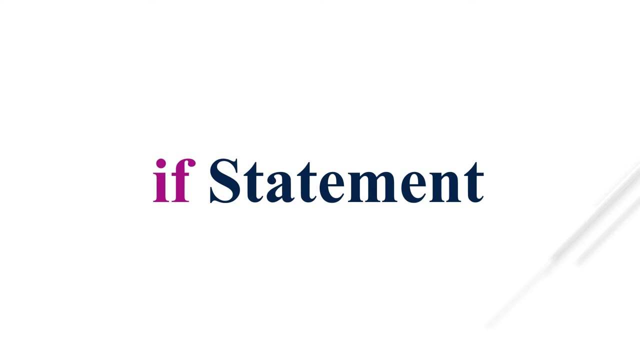 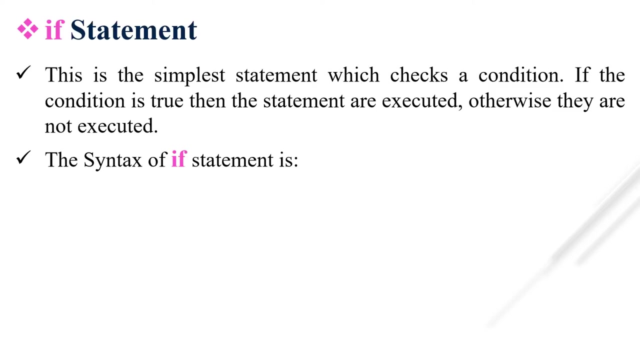 then ternary, then switch and then we proceeds with the unconditional branching. okay, so first we see this part conditional branching, so decision making, and branching is also known as decision making statement or control statement. so the first statement is if statement in conditional branching. now, what is if statement? if statement? this is the simplest statement, which 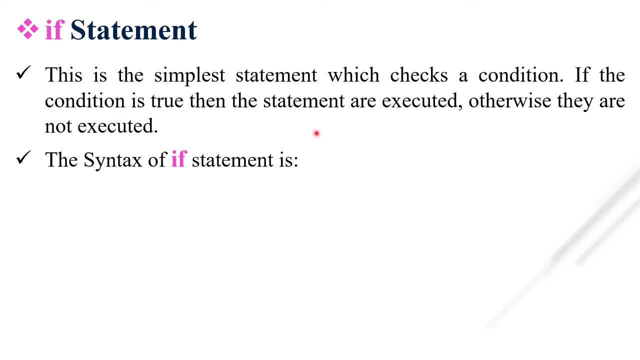 checks the condition. if the condition is true, then the statement are executed. otherwise they are not executed. what is the syntax of if statement? simple, we have to write if in the bracket there is an expression for testing. if it is true, then statement block will be executed. otherwise rest of the program will be. 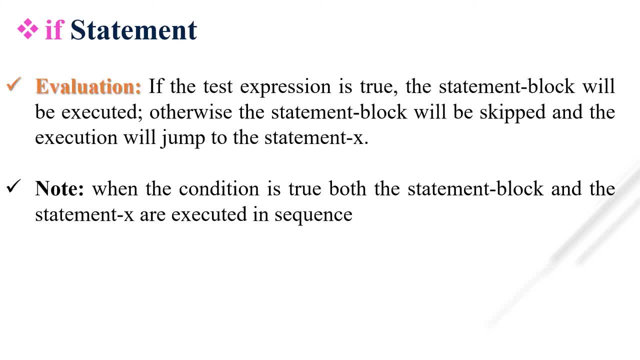 executed. so how evolution is performed in if statement. if the test expression is true, the statement block will be executed. that I already told you earlier. otherwise the statement block will be skipped and the execution will jump to the statement X. 0.3 K accusations caused by the statement block of statement X. 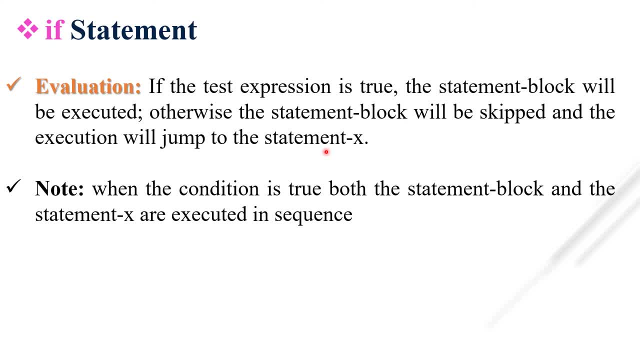 means rest of the program which exclude if statement: okay, if statement: get Bahad Robin huger. that is our statement. X note: when the condition is to both the block, a statement block, and the statement text are executed in sequence. if condition is true, then the statement, the truth statement- okay, if condition is. true, then statement block will be executed. also, statement X will be executed. okay, so here is a simple Hagga été, our real statement unit there, no actual block element. however, if you- if you, they do- come here and read out the statement does, then is that you haszinho if statement, because which means that if we consider this statement is true, then the statement does the statement in legalnego. 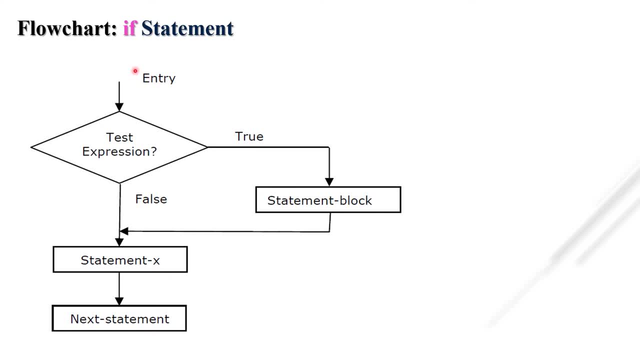 flowchart of: if statement okay we entered, then there is in test expression: if it is true, then that particular block will be executed and then rest of the statement is executed, and if it is false, then this statement is not going to be executed. okay, directly, statement x will be. 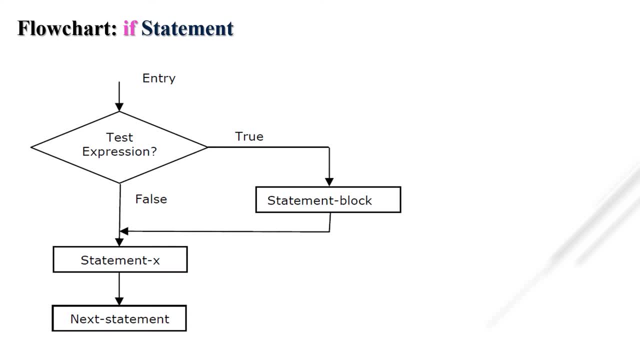 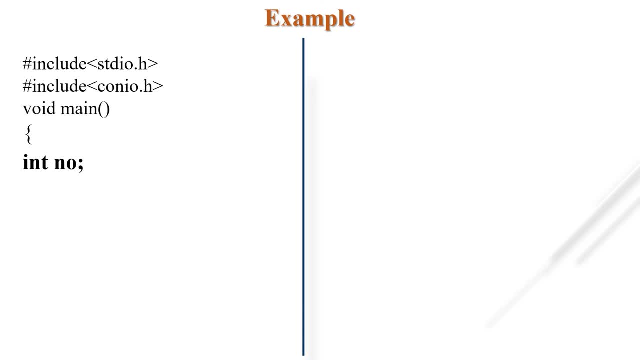 executed in the next statement. so this is an example of if statement. i have taken here one variable whose data type is integer, then we take one number from user side. that's why we are using scanner. a number is stored in this variable, ano, okay. and if that number modulo 2 is equal to equal to 0, then we can say that given number is even. 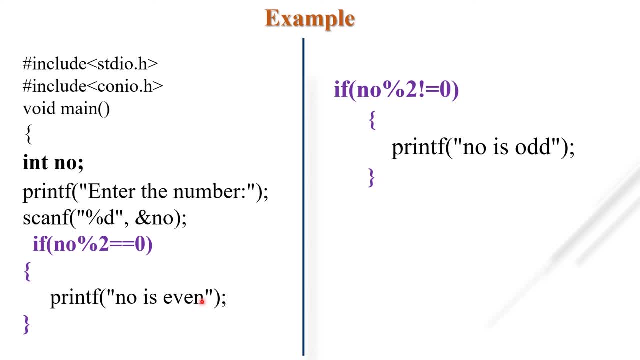 else. sorry, else is not there because we are only looking for if statement. okay, and if n modulo 2 does not equal to 0, this is relational operator. huh, equal to, equal to does not equal to that we already learn in unit number 2. okay, if number modulo 2 does not equal to 0, we print number is odd. 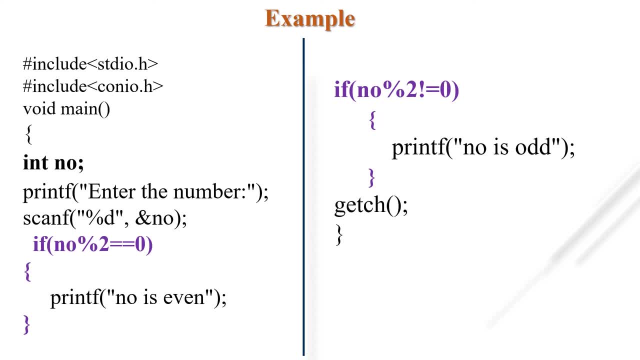 so if i entered here the number 5, okay. so what is the value of this number 5? then your condition will be checked. if 5 modulo 2 is equal to equal to 0, so modulo gives this answer. okay, five modular two, two twos of four, what is reminder? okay, this is the answer for any modulo. 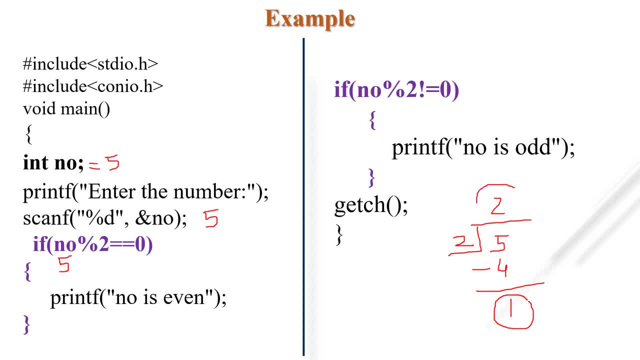 okay, the reminder. if we perform division, then this will be the answer. okay, so if n number modulo 2 equal to equal to zero condition false because number modulo 2 is equal to 1 condition is false, then this part is not going to be executed. okay, so, after this if statement, what is our next statement? this one, okay now. 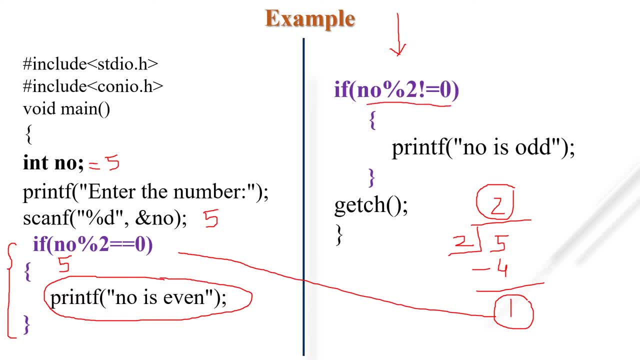 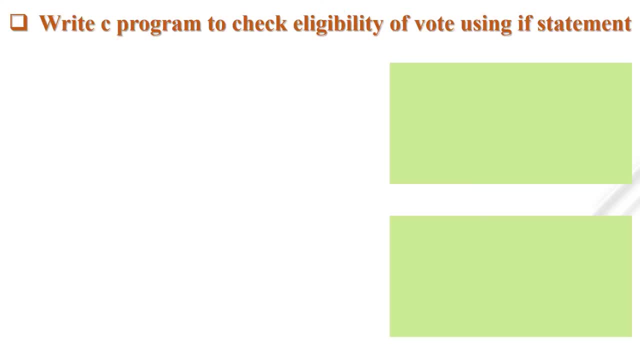 here we check if number modulo 2 does not equal to 0- yes, it is does not equal to 0- then we simply print: number is odd, okay. so here is an another example of if statement. write a c program to check eligibility of vote using if statement, as we all know that eligibility of voting is 18 years. 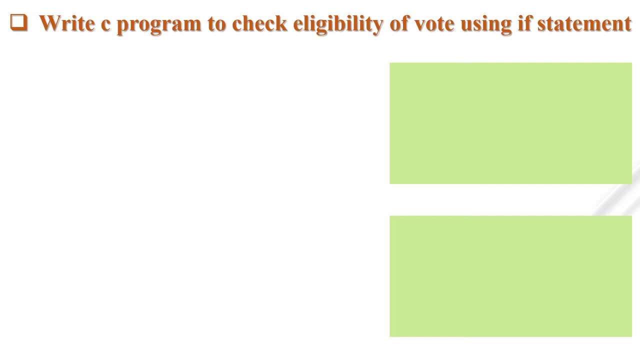 completed, okay. so if the age is 18 or more than 18, then i will. i am eligible, eligible for voting, otherwise not. okay, you. so let do the coding here. i take one variable whose name is age. then user enters the age and it will be stored in age variable- age. suppose i entered 18, 17. next, if age is greater than or equal: 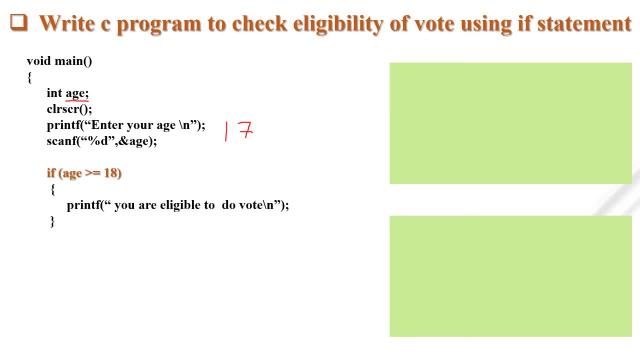 to 18, then you are eligible to do the vote, but here your condition is not fulfilled, okay, so once again, i write: if your age is less than 18, then you are not eligible to do the vote. this will be printed, okay, and this is our statement x. okay, this will be always executed. now what will happen? 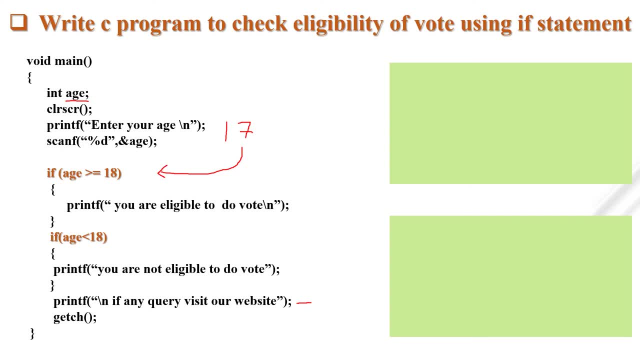 i entered age 17. okay, this condition is false. so this is not going to be executed now, for this is this if statement, what is my statement? x this one. so now this one will be executed here. we condition will be met. okay, 17 is less than 18 condition, true, then compile of a print. you are not eligible to do the vote. 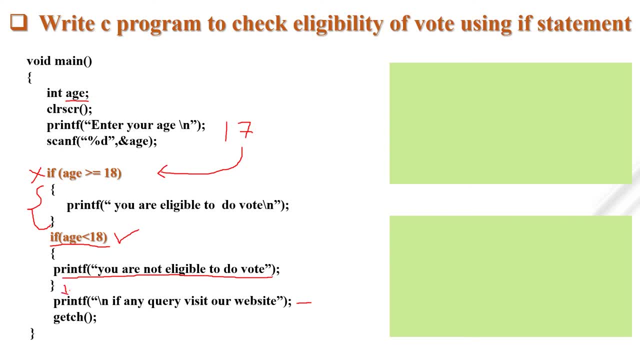 and then this: this will be printed if any query visit our website. this is our statement x. after this, in sequence, this is also going to be executed. okay, let's see what's the output. enter your age- suppose i entered 30- then it will be printed. you are eligible to do the vote if any query. visit our website, because this is our statement x. 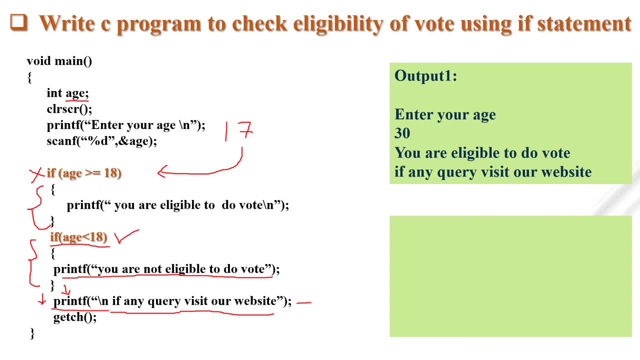 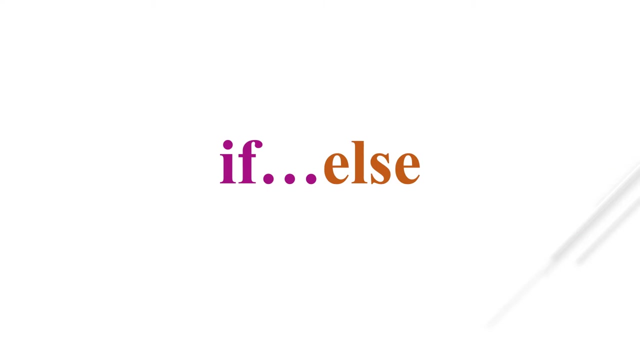 if both condition is all in. if both condition is false, then also this is going to be printed. okay, now second output is: enter your age. suppose i entered 15. you are not eligible to do the vote. if any query, visit our website. visit our website website. So the next statement is, if else, First one is only if statement. Here there is one more. 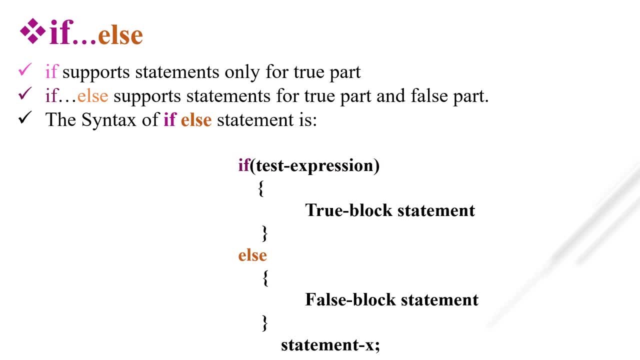 statement that is else If and else. So if supports statement only for true part, Okay, it supports only statement for only true part. This if. But if else supports statement for true part and false part, Both. What is the syntax If there is a test expression? If this condition is true, then this: 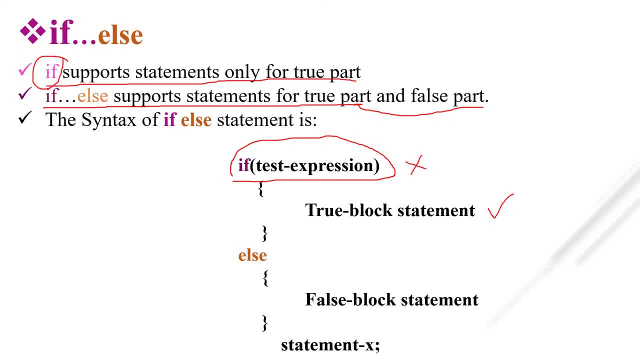 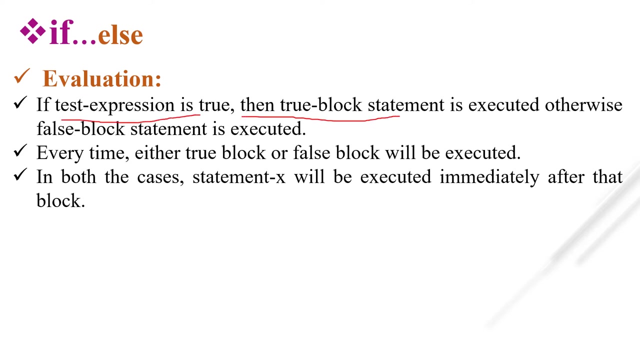 block will be executed. If this condition is false, then this block will be executed. Okay, and then the statement x- that is our sequence of program- That will be executed next. Okay, So how evaluation takes place in? if else, If test expression is true, then true block statement is executed. Otherwise, false block statement is. 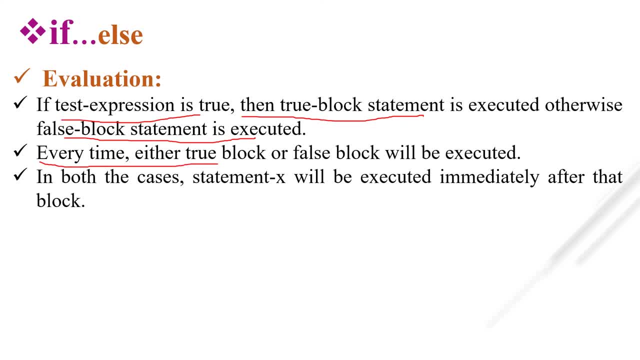 executed. Alright, Okay, Every time either true block or false block will be executed. But in, if only. if it is true, then, and only then, the particular block is going to be executed. If it is false, then there is no block for execution. Okay, But in if else. every time, either true block or 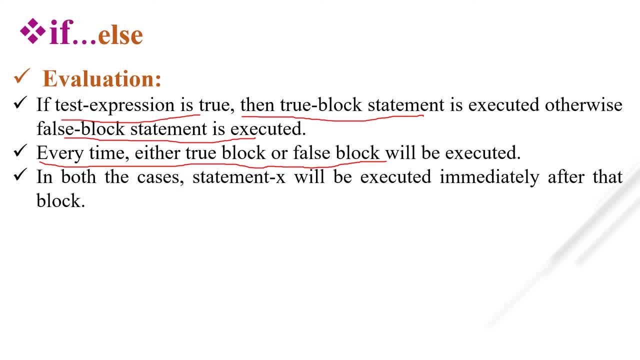 false block, depending on the condition, will be executed. So in both the cases, statement x will be executed immediately after that block. Okay, After if else block, statement x will be executed. I already told you that statement x is the rest of the program. after if else, statement Okay. 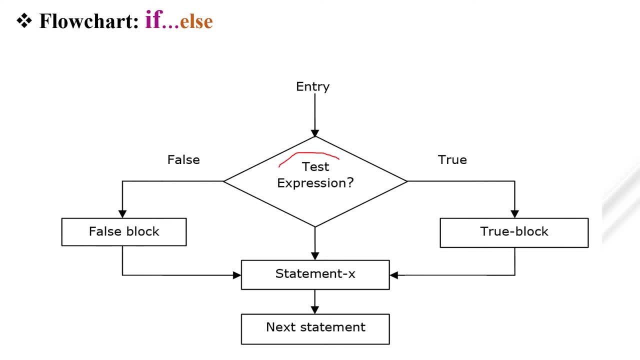 Now this is a flow chart of if else statement. If test condition is true, then true block will be executed. Otherwise, false block will be executed. Okay, Depending on the condition, either false block or either true block will be executed in if else. But it is not true for simple if Okay, And then. 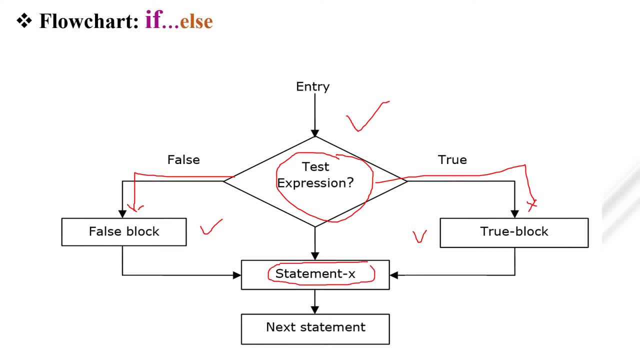 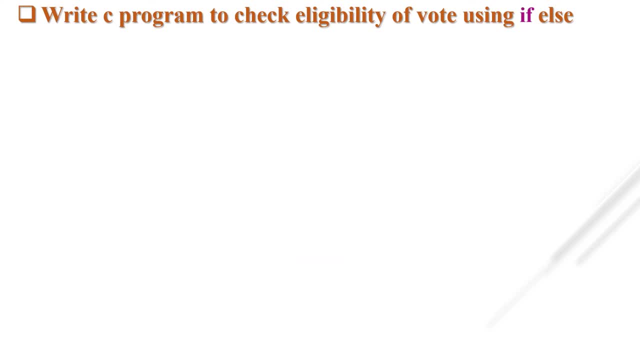 statement x- that is, our rest of the program- will be executed, and then next statement. Let us see the example Here also, I am taking an example to check the eligibility: Like a bö'd, use his browser to check the eligibility of vote using if else. 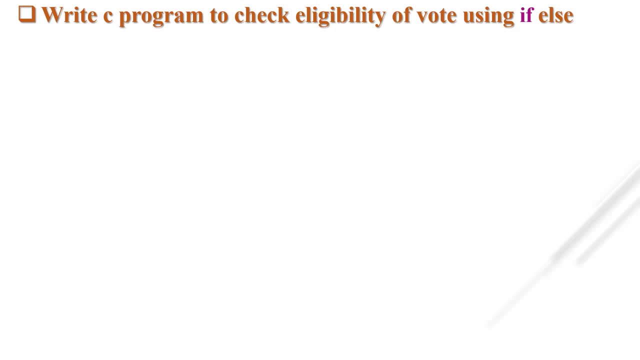 Okay, Let us see the difference of if and if else. Let us see the difference of if and if else. Here also, I take one variable whose name is age. Here also I take one variable whose name is age. User will enter the number. Then number will be stored in variable arm. 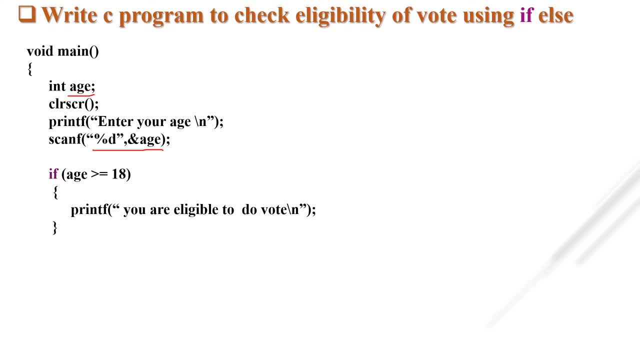 If age is greater than or equal to 18 in your eligible for what? here we have an else. if this condition is not true, okay, then this will be printed. that is, you are not eligible to do the vote. you don't have to write if. condition, once again, that we are all, that we are writing in if statement. 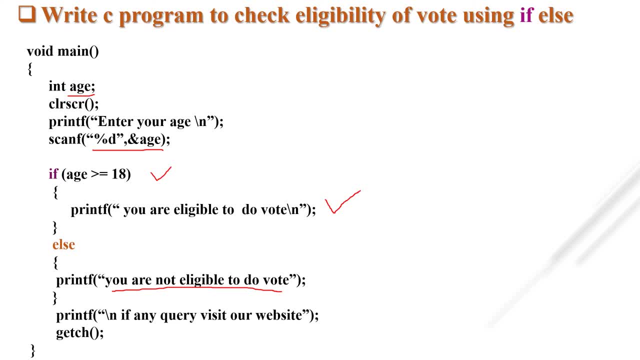 statement X, that is, if any query, visit our website. let's see the output. enter our age. suppose I entered 30 and you are eligible to do the vote. if any query, visit our website. when we entered 30 here, the value of age is 30. okay now. 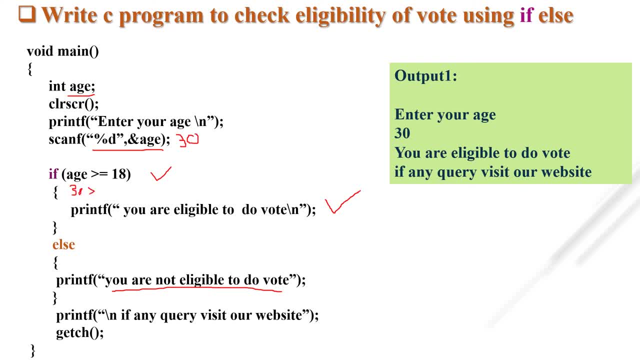 here the condition will be checked: 30 is greater than or equal to 18. yes, it is greater than 18, so if it is true, then this block will be executed. this block is not going to be executed. only one block at a time will be executed in if. 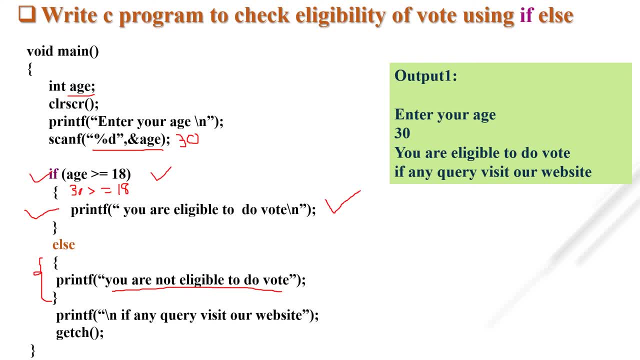 else, either false either true. okay. next is next. output is: enter your age. suppose I entered 15. okay, then what is the value of this age? 15? now your condition will check is 15 is greater than 18. no, it is equal to 18. no condition: false, then this: 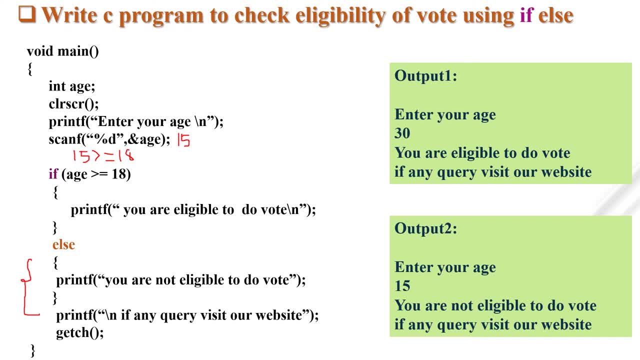 block will be executed, which is our false block. that's why- here what is an output, you are not eligible to do the vote. if condition is not true, then this block will be executed, which is our false block. that's why- here what is an output, you are not eligible to do the vote if. 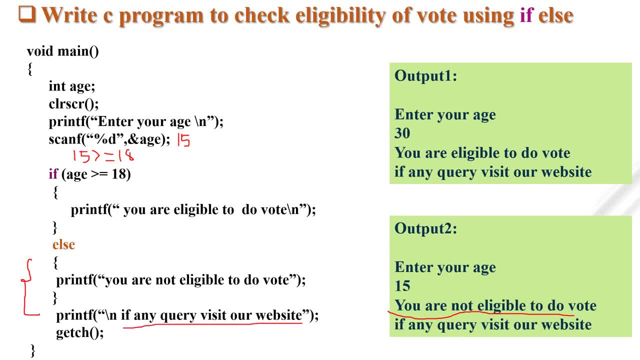 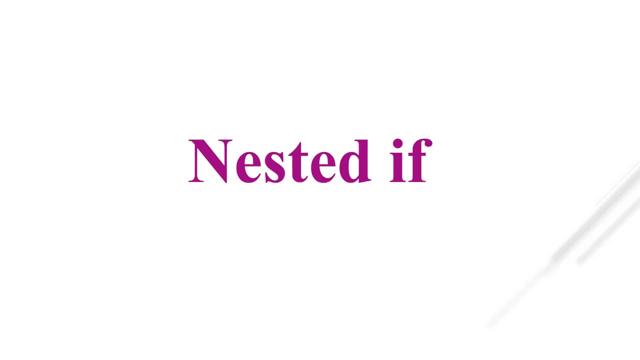 and then, if any query, visit our website. that is our statement x. okay, i think you clearly understand if, if and if else statement. okay, difference between if and if else statement. so the next statement is nested if. now, what is nested if? if we write if statement inside. 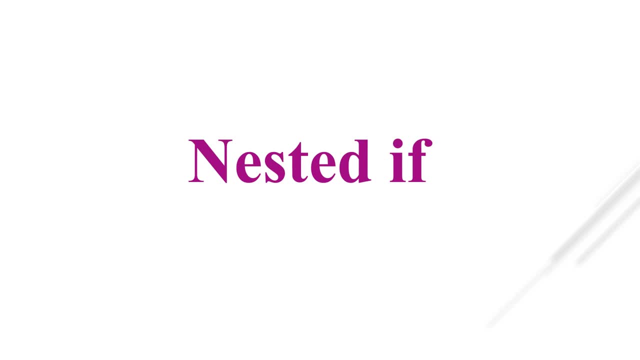 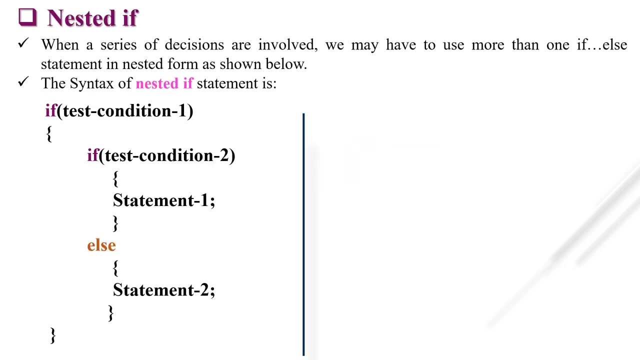 another if statement, it is known as nested. if okay, while checking number of conditions, we may need to nest if statement inside another if statement. that's why it is known as nested. if so, when a series of decision are involved, we may have to use more than one. if else, statement in nested form as shown below. 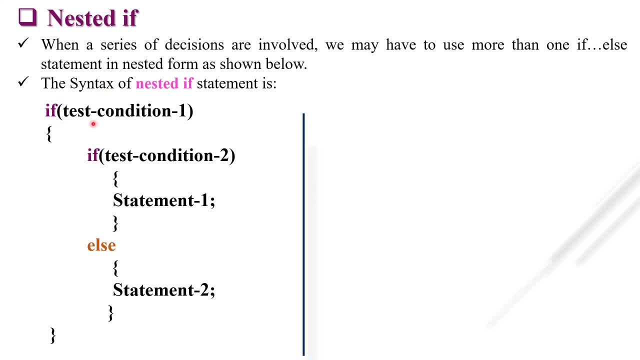 so what is the scenario? so what is the scenario? syntax of nested if: if test condition one, if this condition is true, then second, if condition will be checked, okay, and if it is true, then statement one will be executed, and if it is false, then statement two is executed. now it may be possible: test condition one will be false, then we have to. 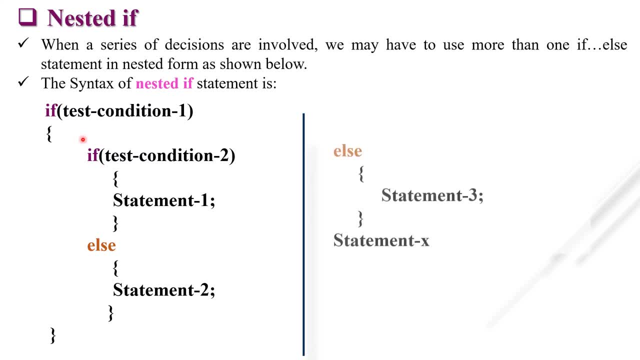 write else part of this. if statement- so here is an else part- then statement three will be executed and then state x. okay, once again i explain you: if this condition is false, then where is the else of this if here? okay, if this condition one is false, then statement three will be executed. 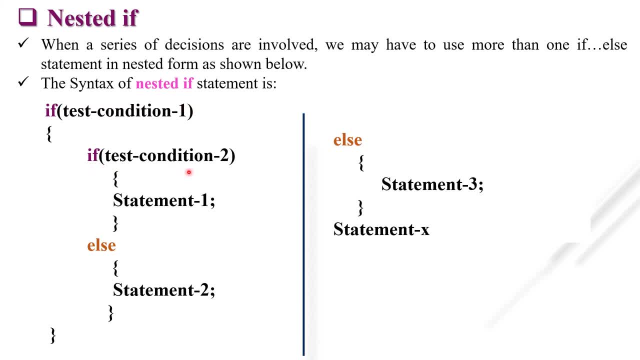 if this condition is true, then we check the condition number two also, and if it is true, then statement one will be executed, and if it is false, then statement two will be executed. okay, and if this condition is true, then there is no need to execute statement three. okay, either statement one. 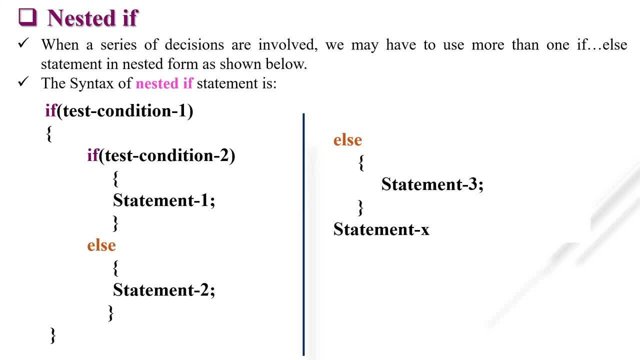 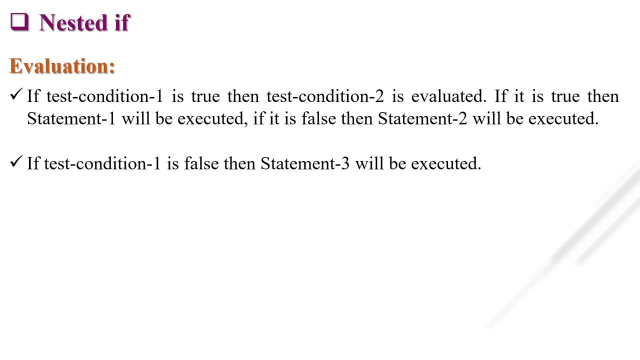 and or statement two will be executed if test condition one is true. okay, so here is an evaluation of nested if: if test condition one is true, then test condition two is evaluated. if it is true, then statement one will be executed. if it is false, then statement two will be executed if test condition 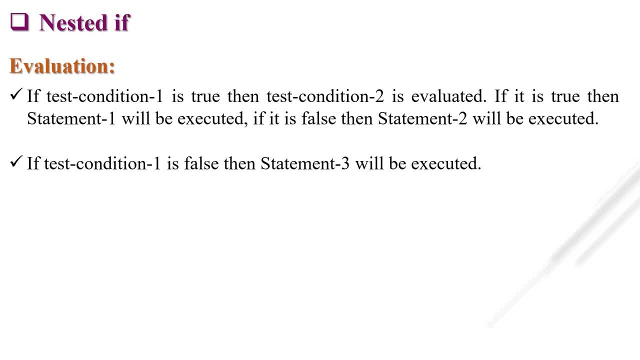 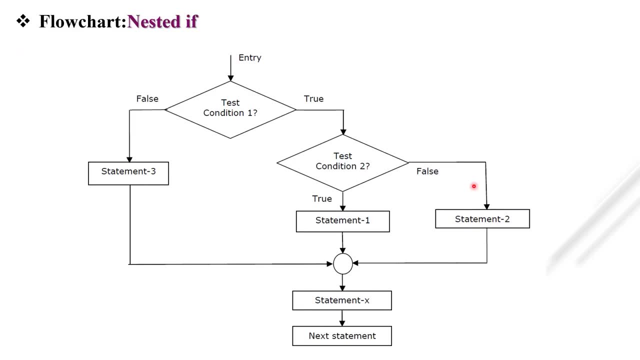 one is false, then statement three will be executed, as i already told you. so this is a flow chart of nested if. if the condition one is false, then directly statement three will be executed. if it is true, because it is an else part, statement three is in the else part. 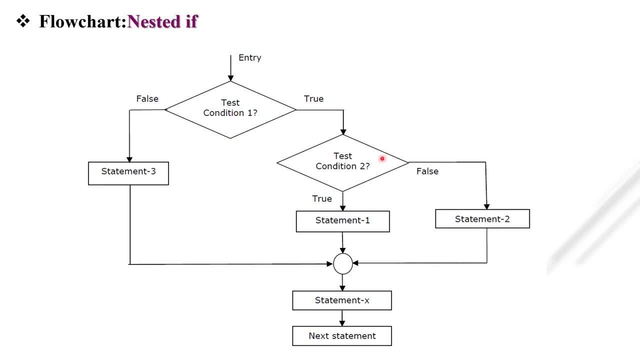 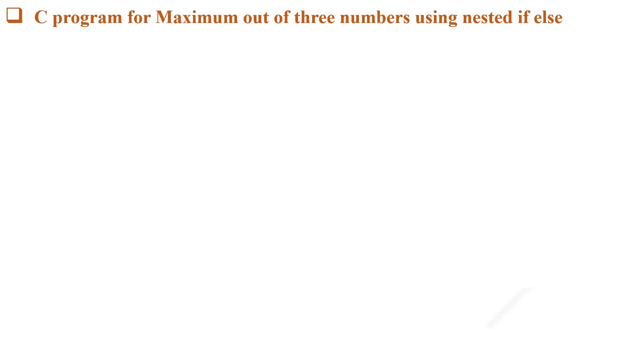 of this statement. okay, if it is true, then next condition will be checked. if it is true, then statement one will be executed, or if it is false, then statement two will be executed. okay, after that statement x will be executed and then next statement. so here is an example where we check maximum number out of three numbers using necessary fields. 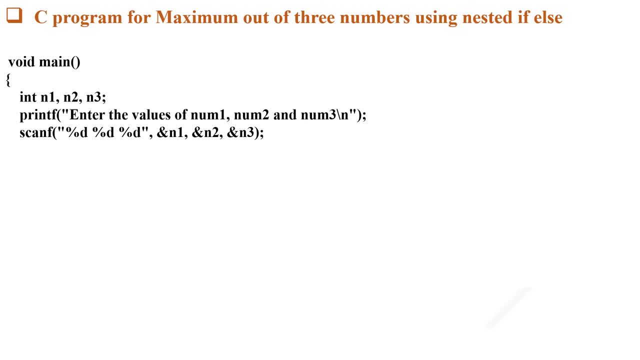 so we have to check three numbers. who is maximum? that's why i have taken three variables: n1, n2 and n3. then user will enter that three numbers using scan up function. then if n1 is greater than n2, then it will be checked with n3. 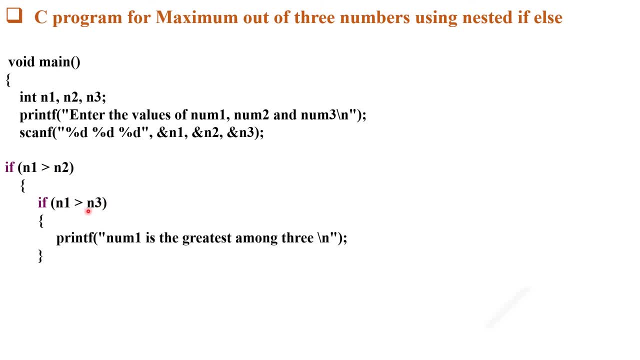 if it is true, then it will be checked with n3. okay, if this is false, then we know that n3 is greatest. okay, i will explain you one by one. and if this condition is false- if n1 is greater than n2, it is false- then directly it is going to the in the else part. 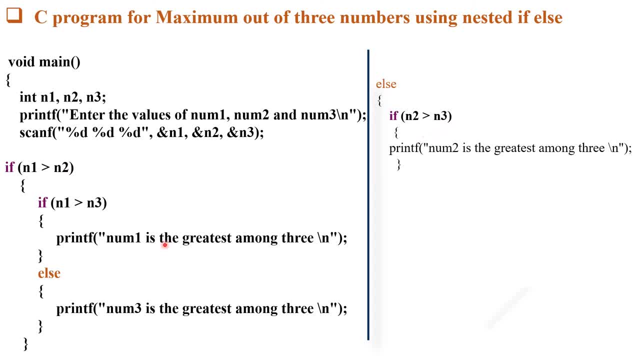 we check once again: if n2 is greater than n3, here n2 is not greater than n1. sorry, n1 is not greater than n2. that's why we checked n2 with n3. okay, if n2 is greater than n3, then n2 is greater. if it is not, then n3 is greater. 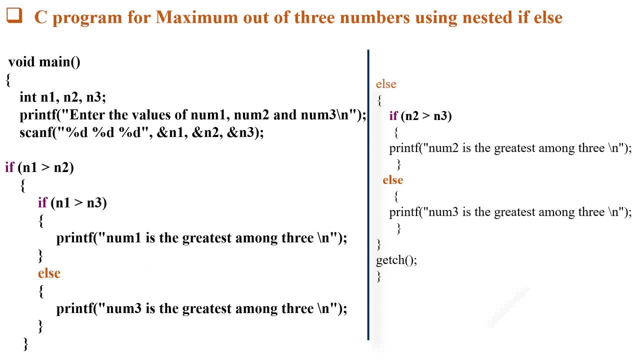 okay, let's check with the number. suppose i entered in number one. one is stored in number two. two is stored in number three. three is stored. okay, we know that three is greater among one, two and three. now your condition will be checked. n1 is greater than n2. what is n1? 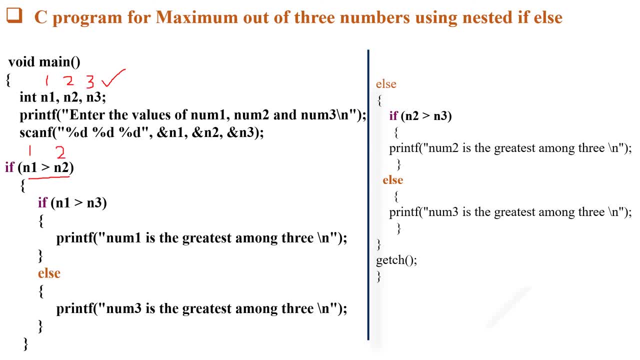 one, what is n2? two, no, it is not greater than n1, is not greater than n2. now the control will directly transfer to else part of this. if, what is the else part of this? if this one- okay, now we check- is n2 is greater than n3, what is value of n2 is greater than n3, what is? 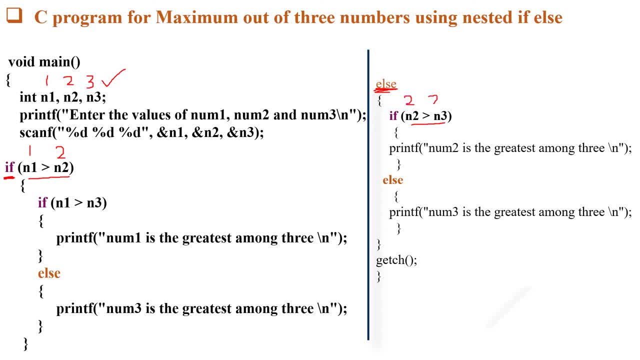 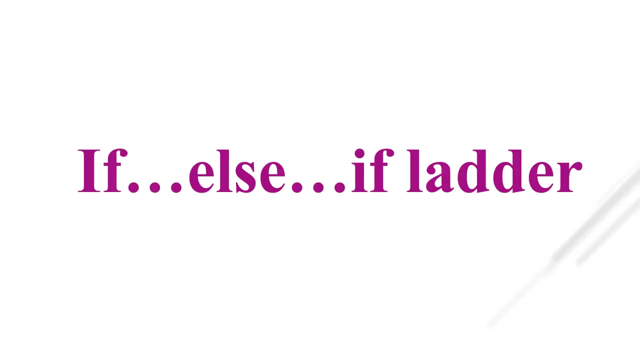 value of n2, two. what is the value of n3, three? no, it is also false. then what is the else part of this, if this one? so what is? uh, what is going to be printed? number three is greater among the three. okay, so next statement is: if else, if later. 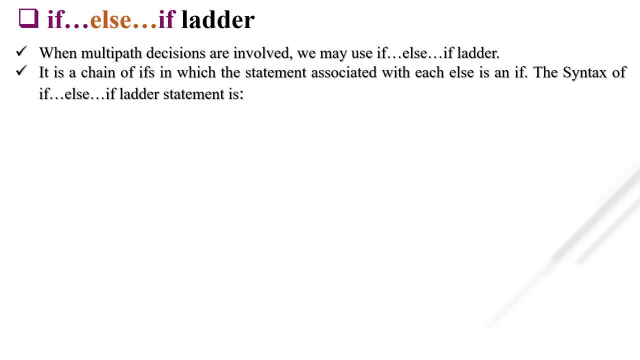 so when multi-path decision are involved, we may use if else if letter. it is a chain of ifs in which the statement associated with each else is an if, so the else if letter is used to test set of conditions in a sequence. it is also considered as multi-way decision making statement. number of conditions are given in a sequence: sequence. 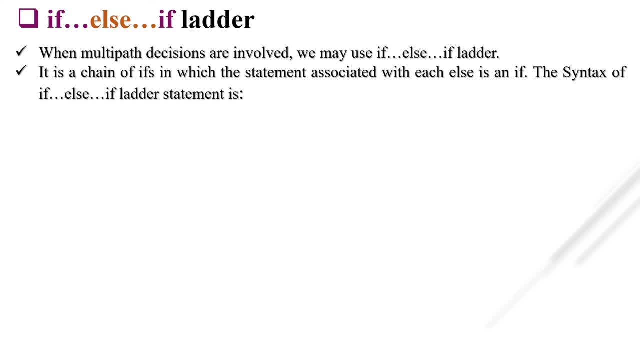 with the subsequent statements: if any of the given condition is satisfied, then the related statement are executed and the control exits from the else if letter. that means further condition are not going to be checked, but if the condition does not satisfy, then the compiler goes to the statement x. let's see what is the syntax of this: if else if letter. 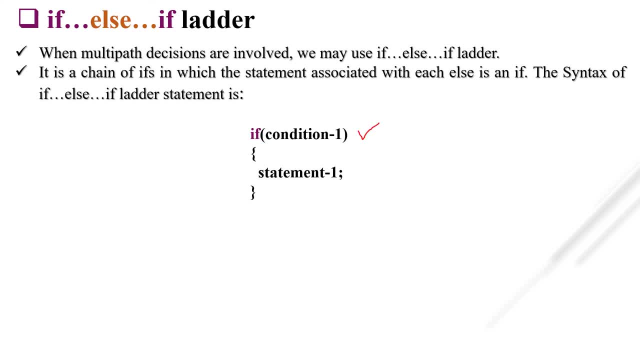 here. if this condition is true, then statement 1 will be executed. if this condition is false, then not else part will be executed in else part. there is another condition that will be checked. if it is true, then statement 2 will be executed. but if it is, 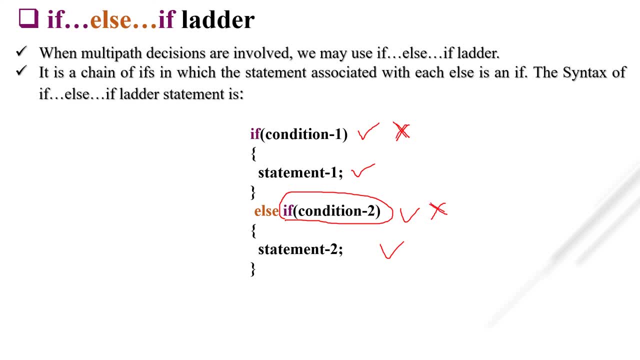 false. if statement 1 is also false, condition 1 is also false. condition 2 is also false, then else, if condition 3, this will be checked. if it is true, then statement 3 will be executed. if this statement is also false, then here i am writing condition, and it may be condition 4, 5, 6, 7, 8, 9, 10. 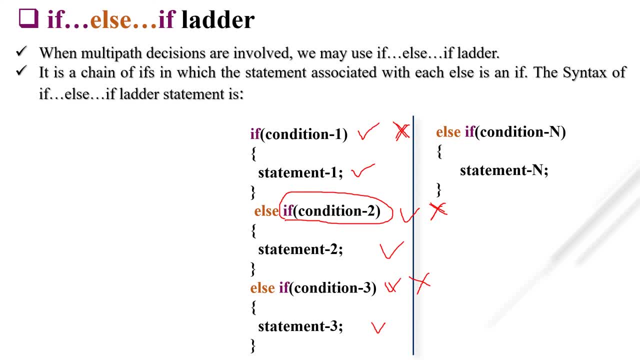 okay, if this statement is also false, then this will be checked. if this statement is true, then statement n will be executed. otherwise, there is one default statement. that condition is not matched in any of the statement. you can use the default statement to writing that statement. okay, let's see one again. if my condition 1 is true, then statement 1 will be executed. 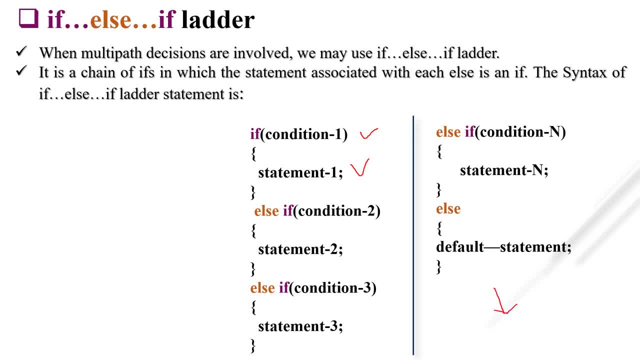 and the control will be transferred to the next statement. these are not going to be executed, okay, but if my this condition is false, so it will be transferred to the else part in that also. suppose my condition 2 is true, then statement true will. statement 2 will be executed. 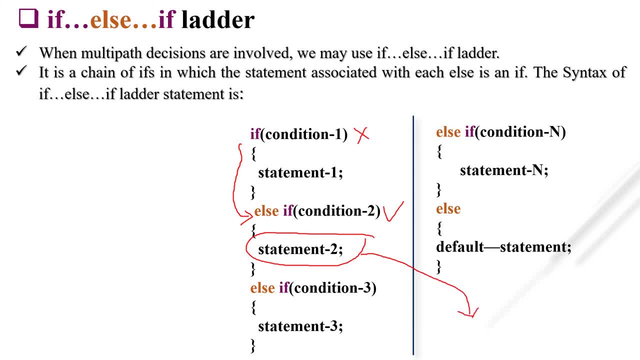 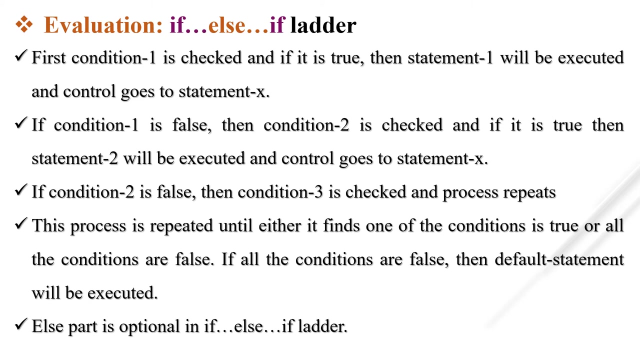 and the control goes to the next statement. okay, this will all are skipped next. okay, so this process repeats until either it find one of the condition is true or all the condition are false. if all the condition are false, then default statement will be executed. else part is optional, else only else part. we are writing for our default statement. 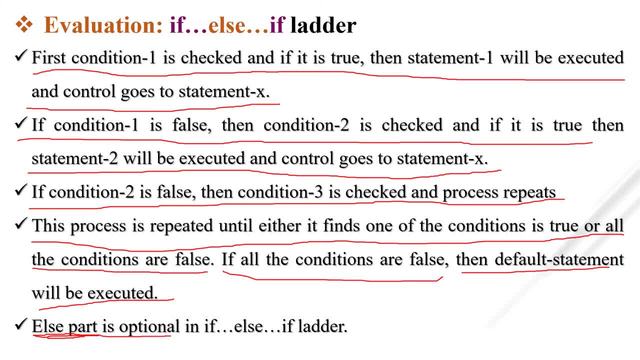 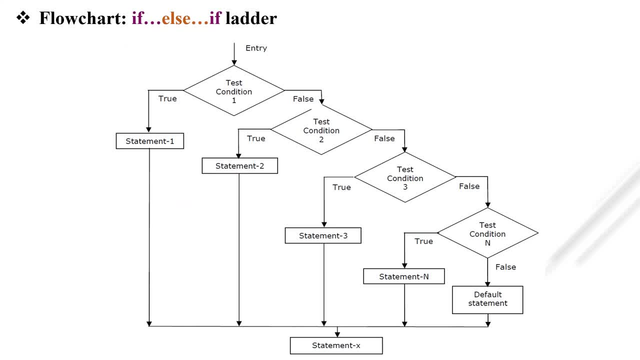 so else part is optional. if you don't want to write, you can. okay, let's see the one of the example. for if else? if leader. so here is an flow chart of IF-ALICE FLADER. if it true, then statement will be one will be executed and directly control will transfer to statement x. and if condition 1 is: 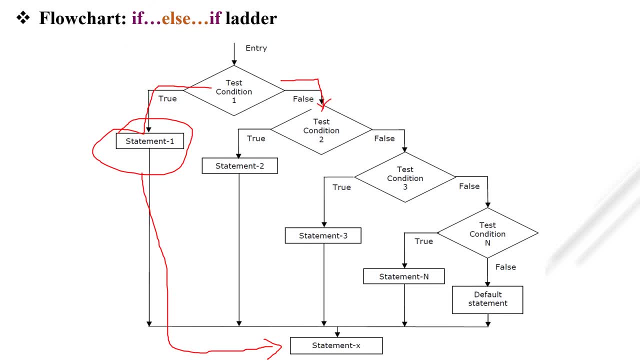 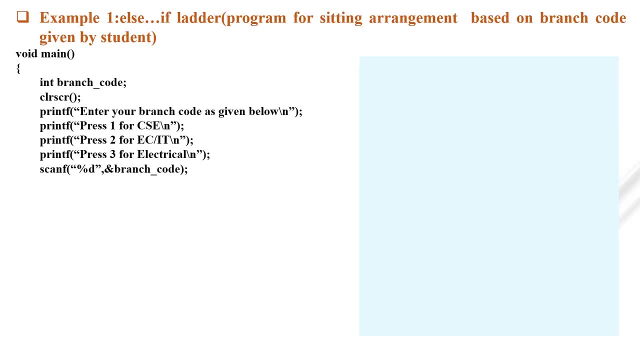 false, then condition 2 will be checked and the process repeats. so let's see an example of IF-ALICE FLADER where we write a program for CTI arrangement based on branch code given by student. okay, so obviously we are only taking from the student branch code, only, okay. so I am taking only one variable. 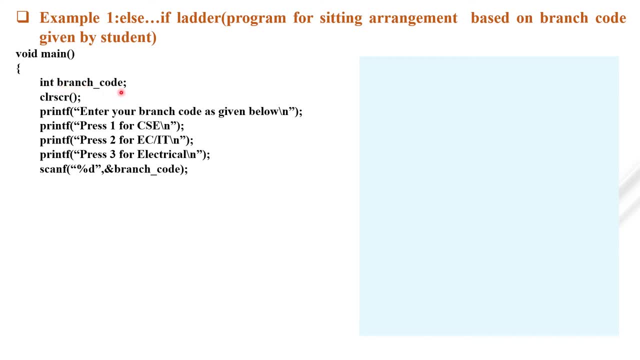 that is branch underscore code. then we print at the output box that enter your branch code as given below: press 1 for CSC, press 2 for EC or IT, press 3 for electrical. okay, now we demand to take the input from the keyboard and it will. 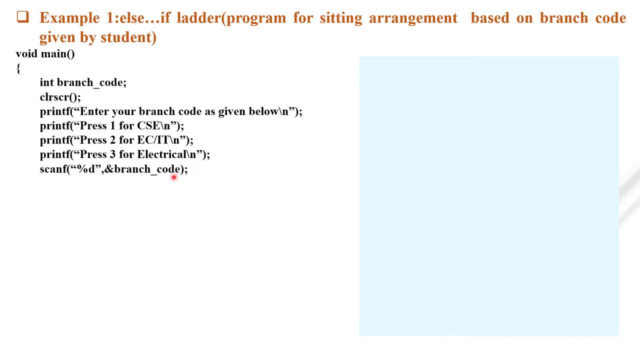 be stored in branch code variable. next we write: if branch code is equal to equal to 1, okay, then we simply printed: go to classroom 02. okay, then else. if branch, Maybe you can print match to available range. better, not, you can have littlebach, because your argument sourced the. 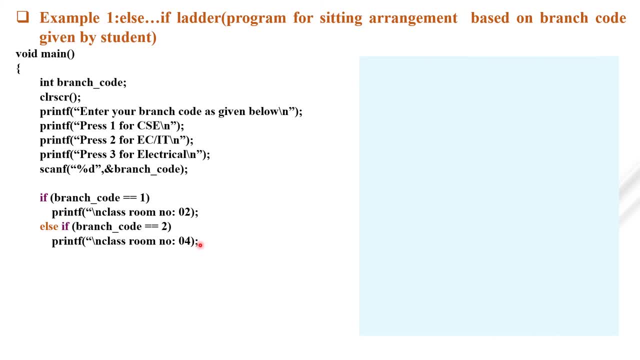 off treatment if entrepreneur goes forecast some. wheremont is not available, electrical, okay. now we demand to take the input from the keyboard and it will equal to two. then go to room number four, else if if branch code is three, then go to class number seven, else this is our default statement: enter proper branch. 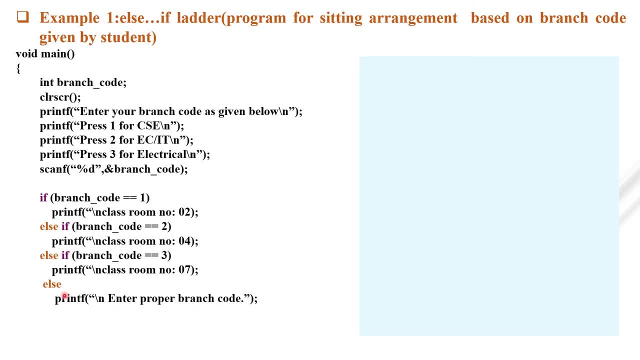 code. okay, so this is an advantage of default statement. if the user are not entering the correct thing, then we can print one of this default statement that enter proper branch code. okay, but this is an optional. if you don't read, then it is also okay. then this is our statement text. that is M jitter. okay, if anyone is. 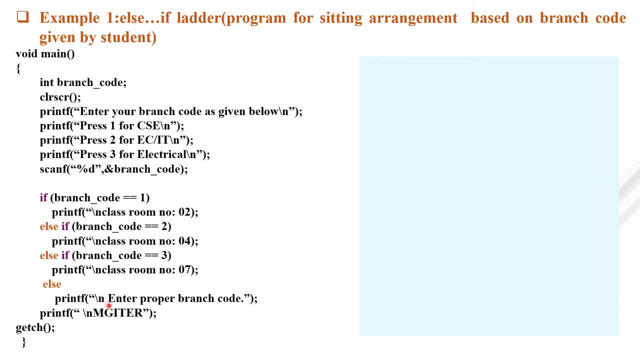 not true from this much, then this two will be printed like: enter proper branch code and M jitter. if I, if user, entered code two in branch code, then condition here it is false, then it will be go in the else part. then once again, condition will be checked if branch code is equal to equal. 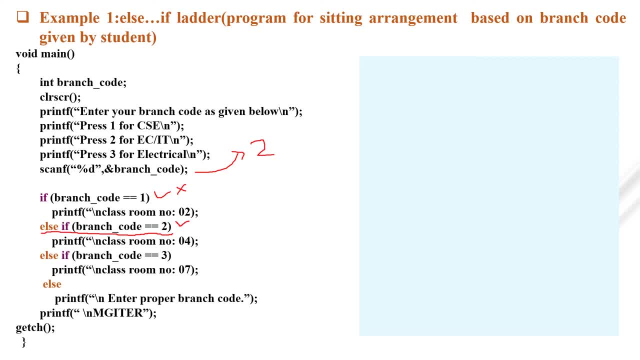 to two years condition. true, then what is printed? go to class number four and it will be exited and directly go to here. then M jitter is also printed at the bottom. let's see the output. if I entered three, then go to class number seven. okay, and then I'm jitter. is our diff data? 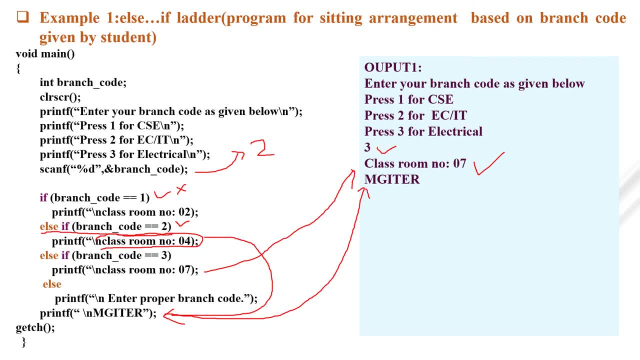 statement x. it will be printed. let's see another output and then the branch code. if I entered one, then this will be true. okay, and this is not going to be executed directly. this part statement text will be executed, that is and jitter. next output. if i write two, then go to class number four and 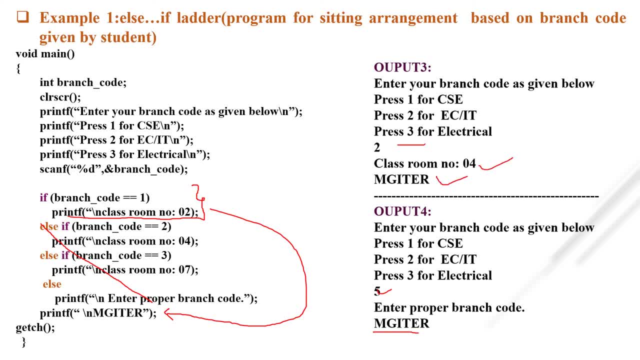 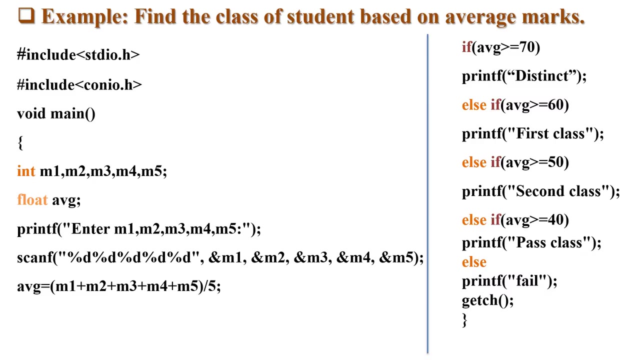 m jitter. and last, if i entered five, then default statement will be executed, because this condition is also false. this is also false. this is also false. then our default statement is: enter proper branch code, and then this statement text will be executed. that is mj okay. so, though, this is an another example of if else, if letter. 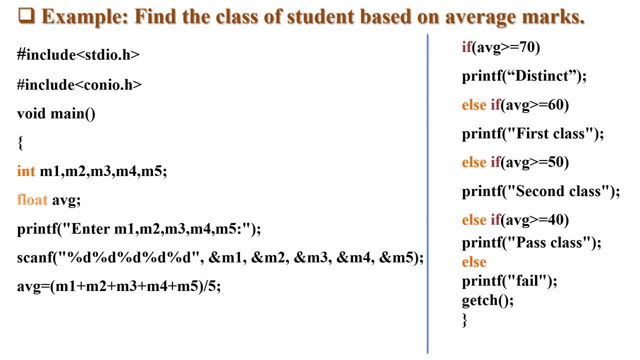 you can try this at home. if you have any query, please contact me. this is very simple. it is for finding the class of a student based on the average mark. okay, if average is greater than or equal to 70, then distinction will be printed. if it is. 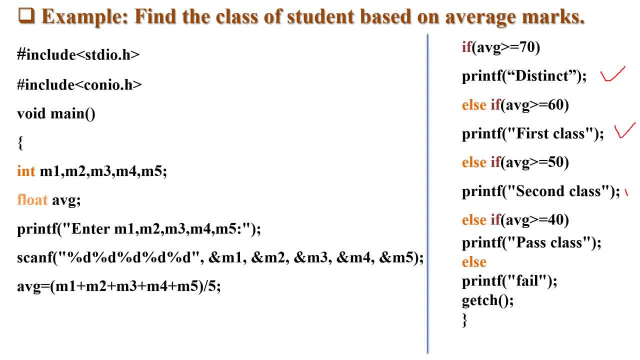 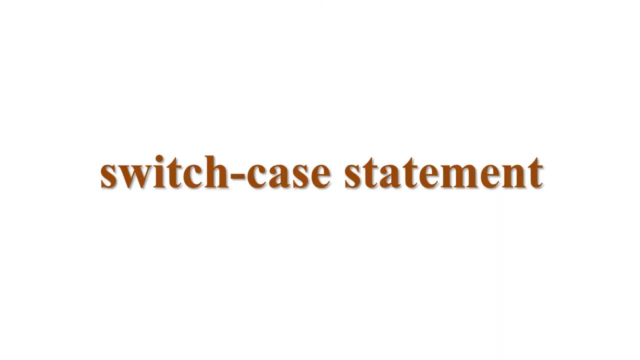 a greater than or equal to 60, then first class 50, then second class. greater than or equal to 40, then pass class, and if our average is 39, then this else part will be printed. it is failed. okay, we can check out. so the next. 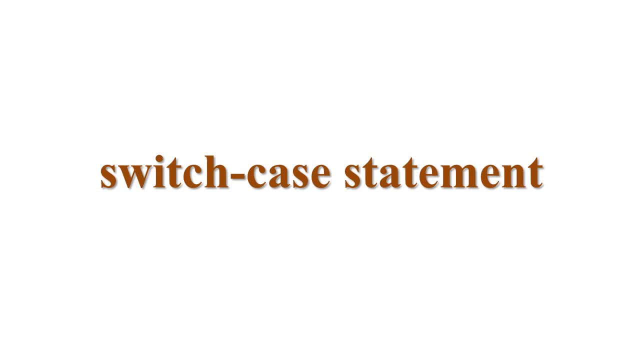 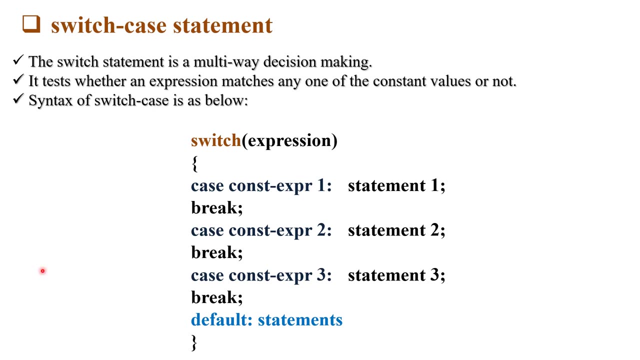 statement is switch case statement. so the switch statement is a multi-way decision making. so it tests whether a expression matches any one of the constant values or not. so there is one constant value we have to match with the constant value. okay, here is the syntax of switch case. 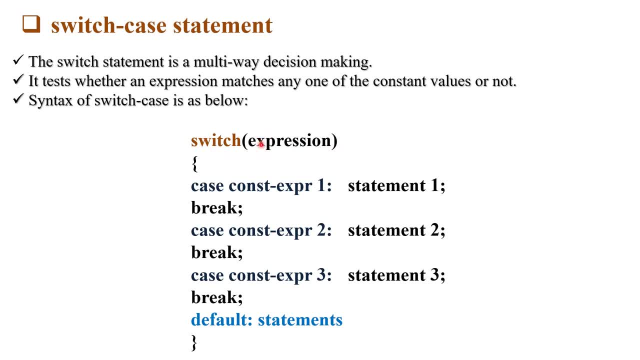 switch in the bracket. we have to write an expression. okay, then case case, then constant expression. you can write case 1 and then colon, case 2, case 3, or you can use a constant, that is string constant, or a character constant, that is a case a, b, c or numeric, simply case 1, 2, 3. 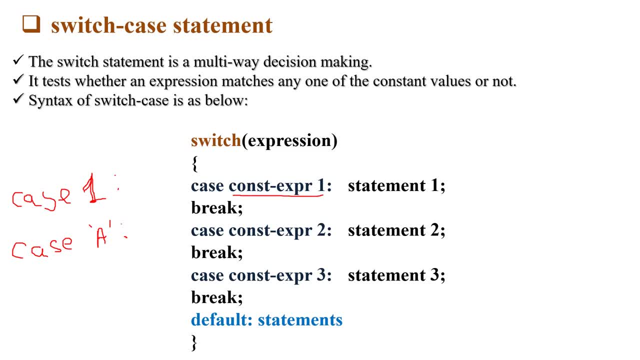 okay, so this is for a, b, c or 1, 2, 3. if you use character constant, then you have to pass one single quotation mark. okay, so this is for a case 1, case 2, case 3, and here also there is a default statement. it is also: 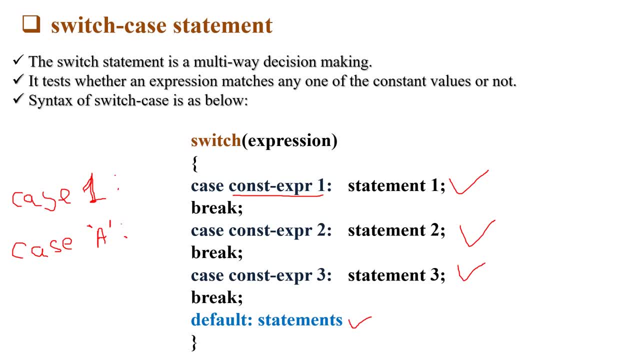 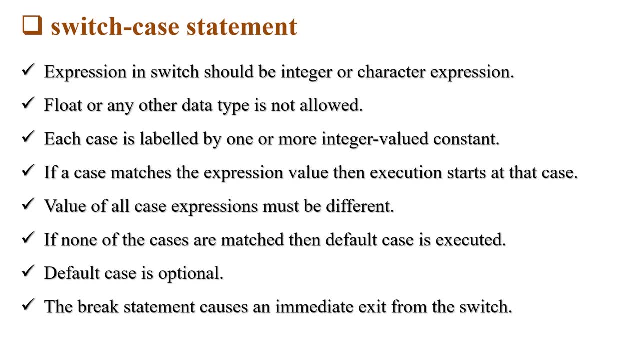 optional. if you want to write, you can. otherwise it is not necessary. let's see the explanation of this switch statement. so expression in switch should be integer or character expression. float or any other data type is not allowed. this is most important. float or any other data type is not allowed. only integer and character will be allowed. 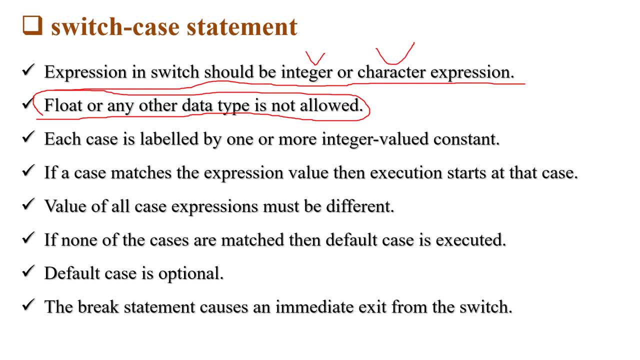 okay, each case is labeled by one or more integer value constant. okay, that i already told you that case one. okay, this is an integer value constant. integer value constant or you can write character in single code. it is also constant, character constant. so if a case matches the expression value, then execution start at that case. 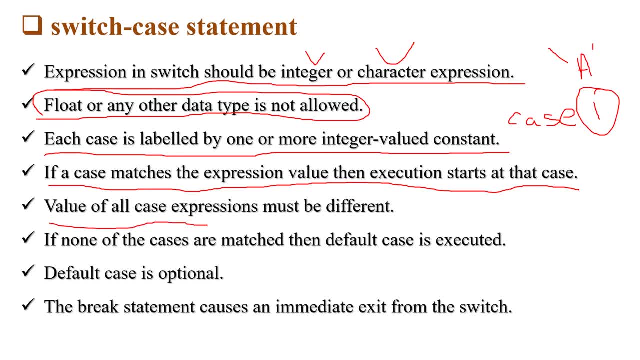 values of all cases. expression must be different. okay, if i use case one, then i must have to use case 2, case 3 or case 100, case 55, but this will be unique. okay, if i use case 1, then i cannot able to use. 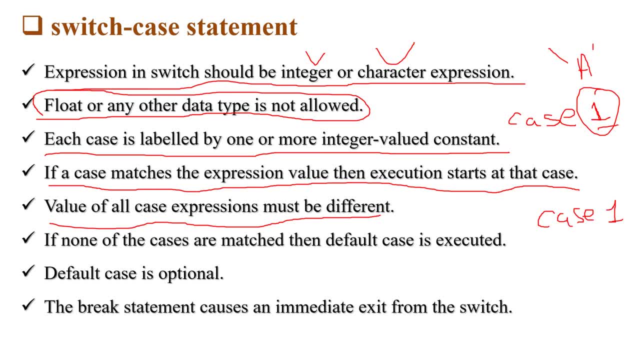 another case one. okay, it must be different. if none of the case are matched, then default case is executed. default case is also optional here and the break statement causes an immediate exit from the switch case. okay, now, what is the role of this break statement in this switch case? i will 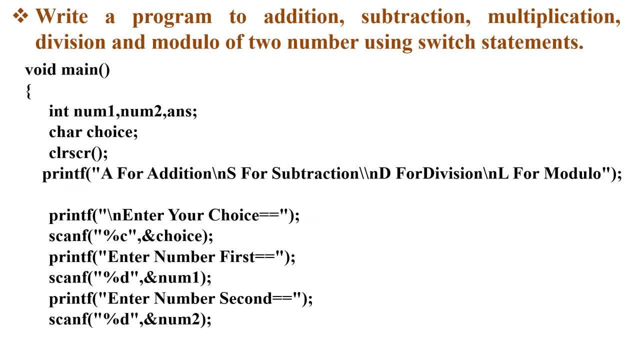 explain you in next slide. so here is an example: write a program to addition, subtraction, multiplication, division. so here is an example: write a program to addition, subtraction, multiplication, division and modulo of two number using switch case. okay, so i take two number in integer in the data type of number, and num two is integer. 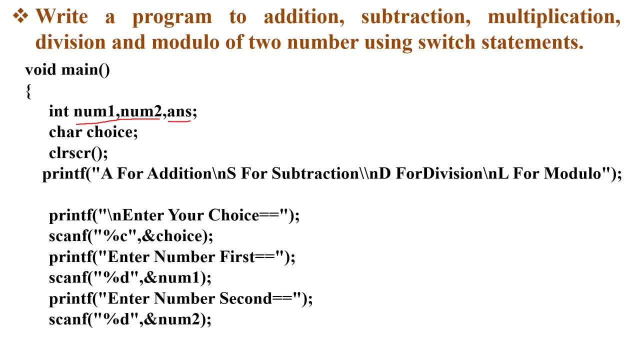 and the variable answer is also have the data type integer. okay, whatever we store, we are storing. in answer, then i am taking character, the is channel data type and so physical number in integer character constant which is stored in choice. so in choice variable we can store a character constant. 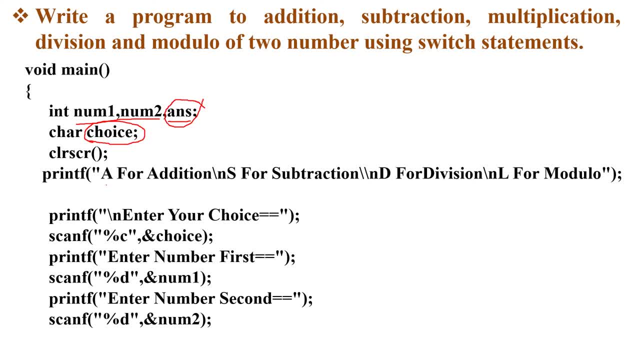 okay, then i simply printed that: press a for a for addition, s for subtraction, d for division, l for module. okay, i am not mentioning here multiplication, you can do with your own. okay, now, next, what i ask: enter your choice, what you want to do. they can press either a either s, either d for division or l for module. okay, and it will be. 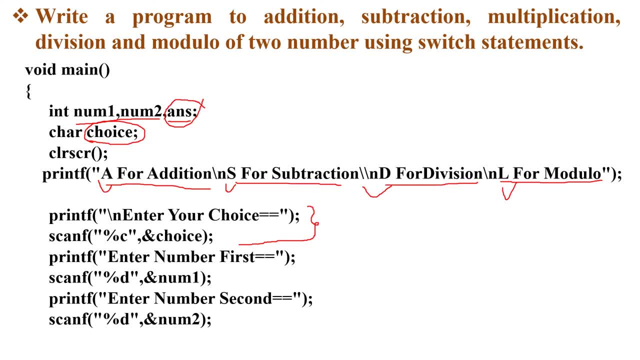 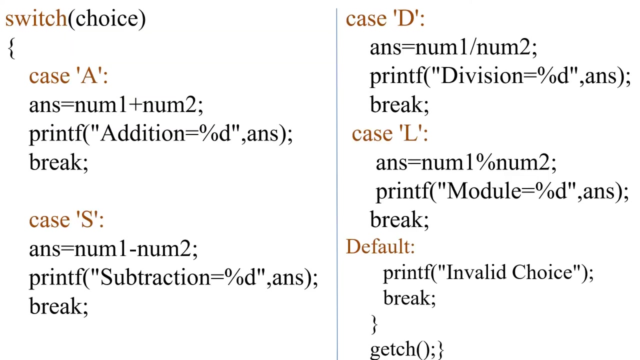 stored in percentage c because we are using character data type, we are using percentage c and the address of that particular variable is okay, in at this address. whatever here we entered will be stored. and then we ask for number one and we are going to store in number one and ask for number two and that will be stored in num2. okay, next switch choice, suppose i. 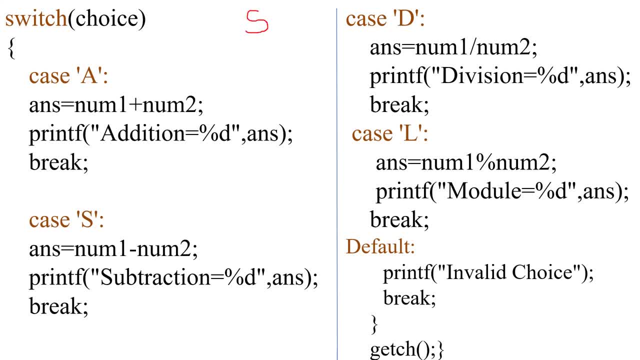 i have a choice s. okay, i entered in choice variable s. then directly, this case will be executed where answer equal to num1 is already stored earlier. okay, answer equal to num1 minus num2 and directly. i printed here: what is the role of this break statement. 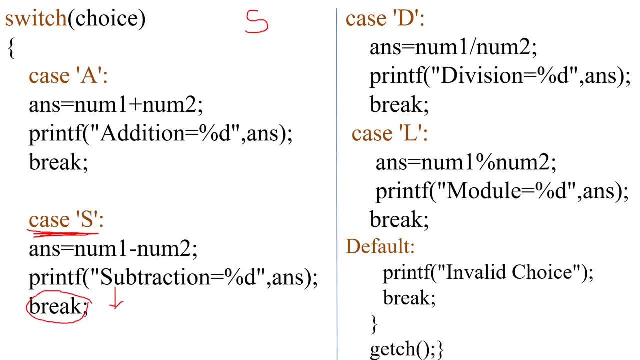 after this, break statement will be invoked. break statement is helpful to exit from all the, from all these switch cases. okay, so after break we are here, it will be exited from the switch case. that's why we are using break statement. okay, suppose i entered d in choice variable. then, directly, this case will be executed. 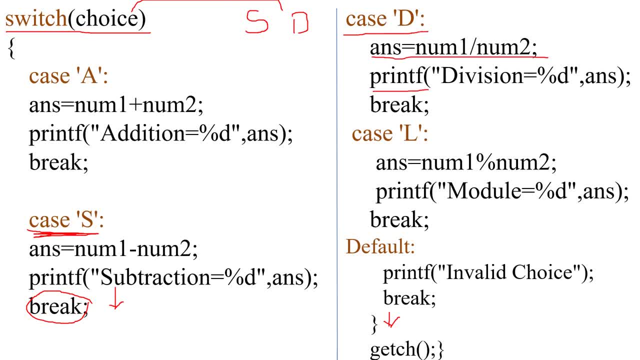 in this answer equal to num1 divided by num2, then division- answer of division will be printed and then break. break means you have to exit from this switch case. compiler know that now i have to exit from this switch case. okay, if i entered z, okay, so this is not case a. this is also not case s. it is also not a case t, not a case l. 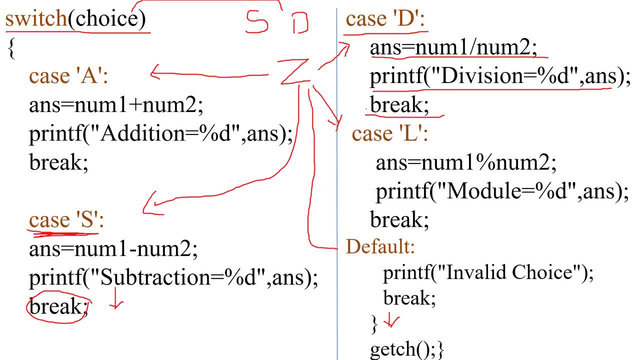 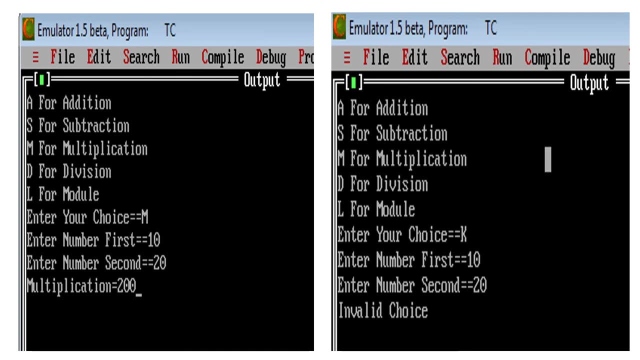 then default case will be printed. that is invalid choice break. okay, let's see the output. okay, so when we press control f9, we, when we run this, our program, then this will be shown to you. then choice will be entered by the user. suppose i entered m, then enter first number. 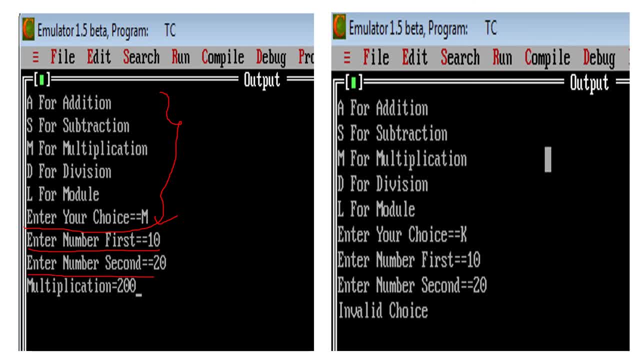 enter second number and directly this m will be executed. where 200 is the answer: okay, it does not have the multiplication coding in our slide. you can type with your own. okay, the second output is if i write k: okay, then also it will be asked for num1, num2 and then. 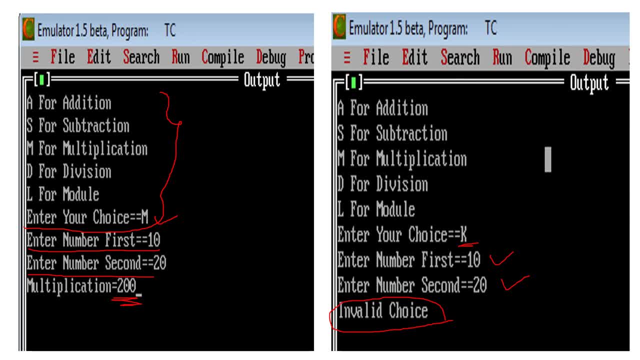 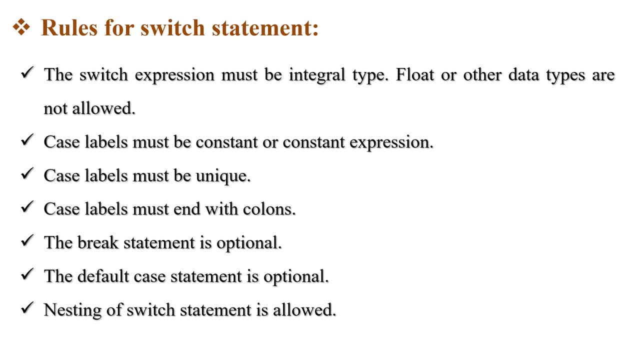 the default statement will be invoked. that is invalid choice. so rules for the switch statement is the switch expression must be in integral type. float or other data type are not allowed. case label must be constant or constant expression. that i already told you. case label must be unique. 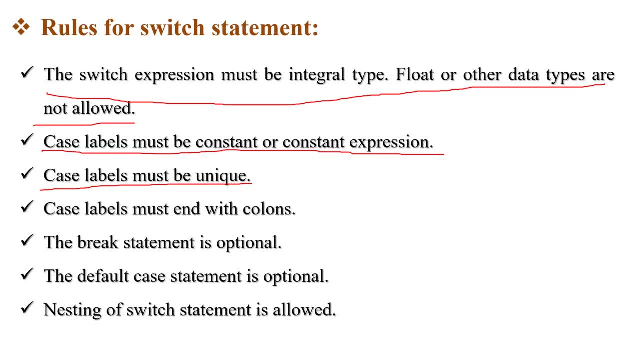 also, i already tell you, told you that case one, case two, case three is three. we are not able to use case three, uh, many times. okay, only one time we can use. case label must be ends with colon. okay, if i write case space one, then it must be end with colon. 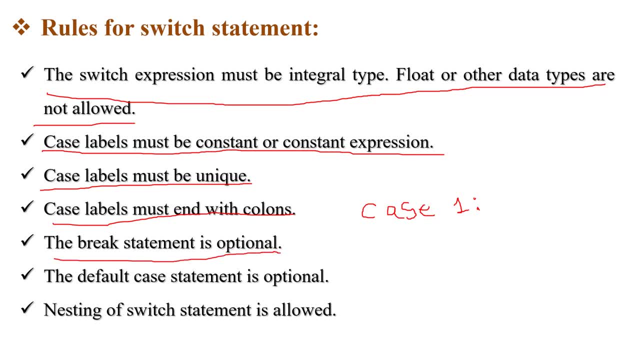 the break statement is optional. if you don't want to break in between, then it is an option. you can not, then you have. you don't have to write this break statement. okay, the default case statement is also optional. i already told you, nesting of switch statement is allowed. okay, next one. 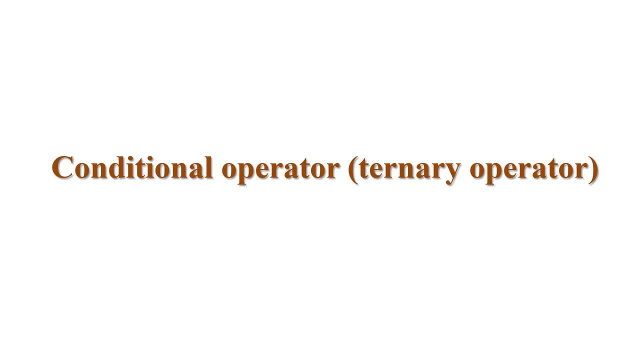 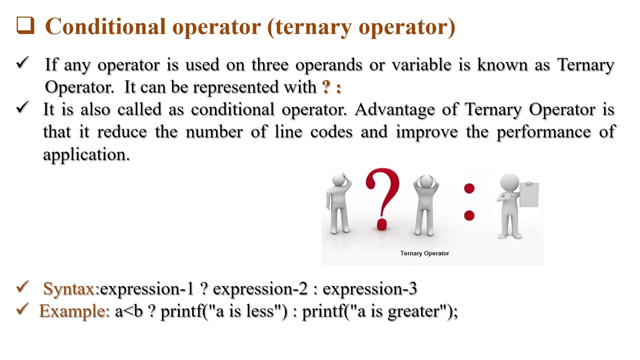 is conditional operator, that is also known as ternary operator. this is also most important statement for our examination. okay, so conditional operator is also known as ternary operator. so what is conditional operator? if any operator is used on three operands or variables is known as ternary operator. it can be represented with this question mark and colon. 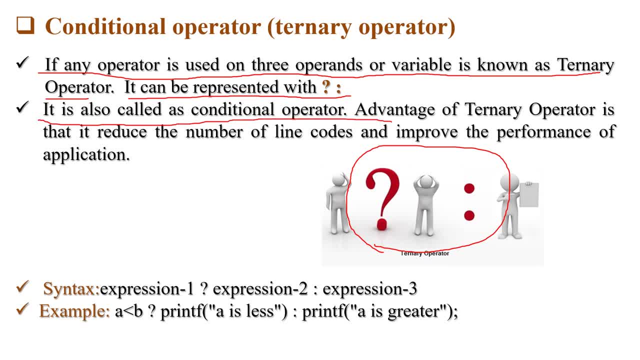 okay, it is also called as conditional operator. advantages of ternary operator is that it it reduce the number of lines, codes and improve the performance of application. so what's the syntax? syntax? we have to write expression one, question mark. expression two, colon. expression three: if this expression 1 is true, then expression 2 will be executed. 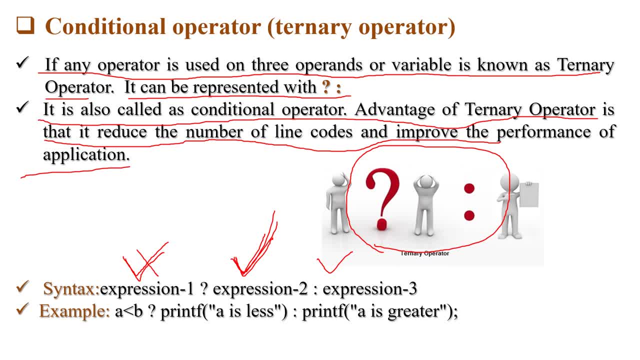 if expression 1 is false, then expression 3 will be executed. okay, here is an example. if expression a is less than b, suppose the value of a is 5 and the value of b is 100, so condition fulfills a is less than b. so what will be printed? a is less. if this condition is false, then, and only then, 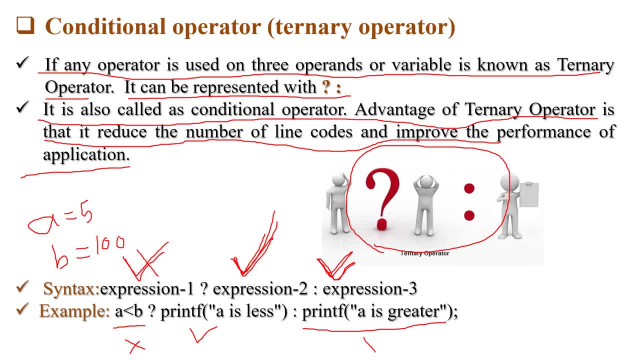 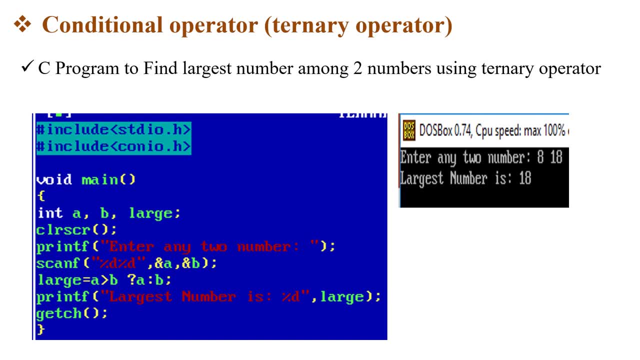 which part will be printed. this expression, 3, that is a, is greater. okay, so this is an example, see program to find largest number among two number using ternary operator. so first we take two variables, a and b, and third variables for storing among these two which one is large. okay, 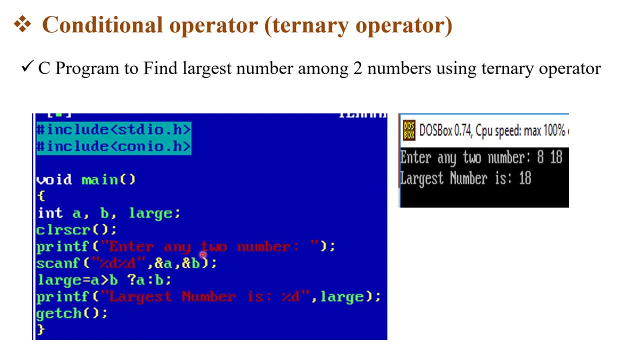 enter any two number, then user will enter two numbers which are stored in a and b. okay, then we simply checked here with the help of ternary operator: is a is greater than b? if a is greater than b, then answer of a answer means the value of a will be allocated to large. 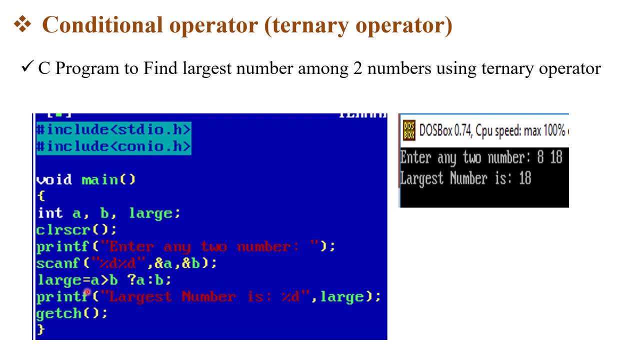 that's it. if a is less than b, then the value of this condition is false. then the value of b is allocated to the large. okay, then we have to print the large, okay. so if i, uh wizard- entered 18 and 18, the value of a is 8. 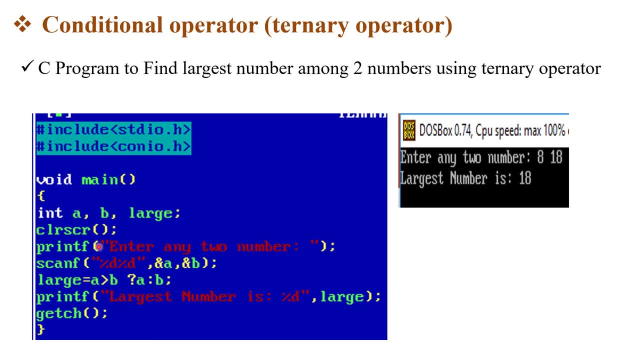 the b is 18. okay, 8 is not greater than b, so this part, expression three, will be allotted to the large variable okay, that's why here printed 18 2018. So the next topic is the difference between if-if-asWorld and sweet statement. so, as we know, if statement is used to select aick-a-dick or to select groupables, you use the imm outstanding. in this case you have often reference statement. but for Wervel, for example, description: oh, you have foreign youngsters, so you use the imm outstanding. in this case, you have. foreign subjects, you use the imm outstanding. in this case you have foreign subjects anyways. now, express a or not BERM problem. you have also many variables. therefore there are some необ and haya in this particular statement. so the most important aspect is to identify and decl. Rick was said, there is some. 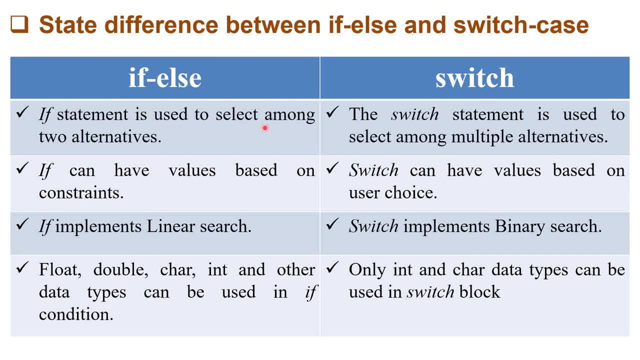 yeah, answer from those that you see like this in facebook: statement is used to select among two alternatives, but switch get statement is used to select among multiple alternatives. okay, we, we can add the alternatives, multiple alternatives, with the help of case case 1, 2, 3, 4, 5, 6, 7, 8, 9. 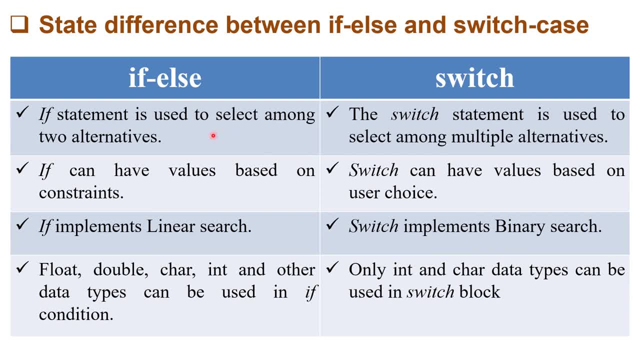 10. but in this if else, only two alternative will be checked. only one of the alternative will be printed. okay, if if can have values based on constraint switch. switch can have values based on user choice. if if implement a linear search, okay, will be linearly searched in. if else, but switch implement binary. 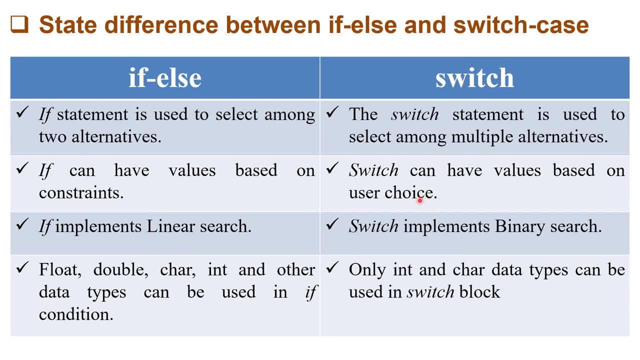 search because of choices. okay, we have a number number of cases. that's why we are using binary search. in switch case, float, double character, integer and other data types can be used in if condition, but in switch statement only integer and character data type can be used in switch block. 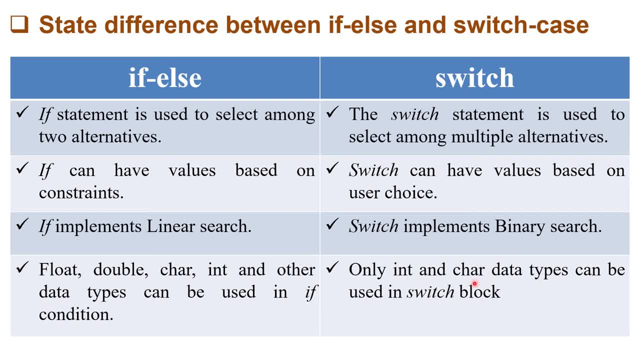 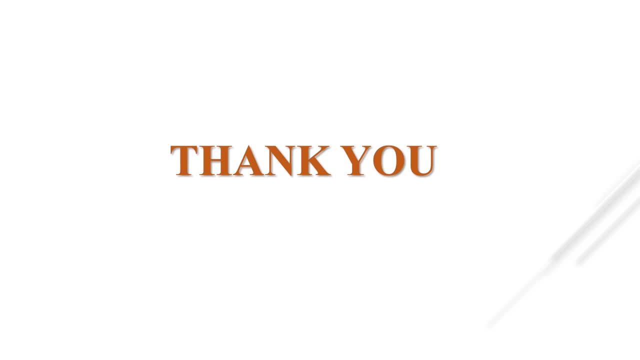 integer like case 1, 2, 3 character. that is our character constant in single code. we have to write case a, case B, case C. okay, hope you all understand the content of the video. if you have any query, please contact me. thank you.